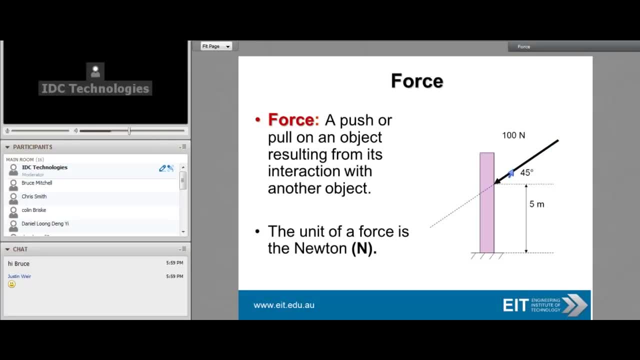 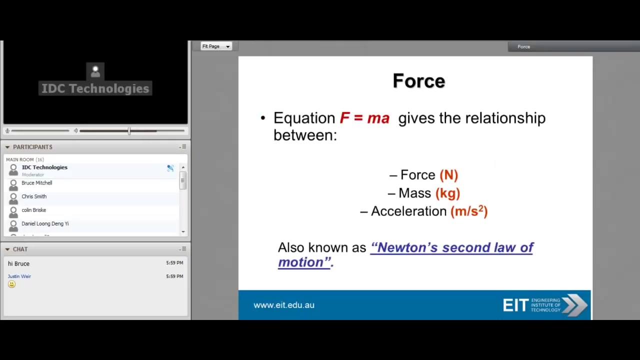 civilizing. and we're applying this to this column at an angle of 45 degrees, five meters from the bottom here. So engineers like to do cool things. so engineers could work out how much this column moves because of this force applied here, And we could even work out things like bending stresses. but not to worry you just now. More about that later. 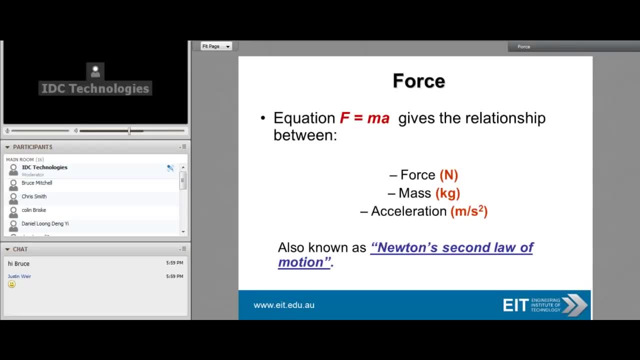 Now, the force is a product from a material, playport, oxalis, product of mass times acceleration, mass being measured in kilograms and our friend acceleration, of course, being measured in meters per square second. And this equation, here F equals mass times, acceleration is known as Newton's second. 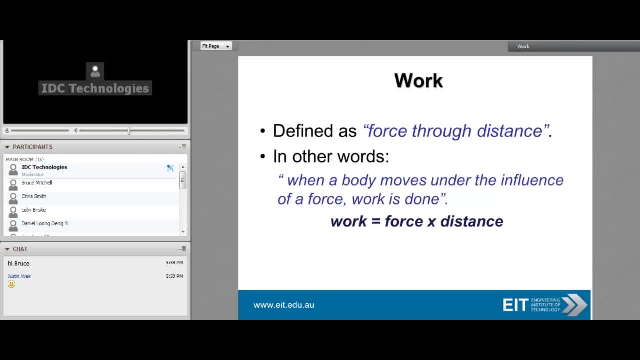 law of motion. If we're going to do work, it means that we have to do or produce a move of force through a distance. So the definition here of work is when a body moves under the influence of a force, work is done. 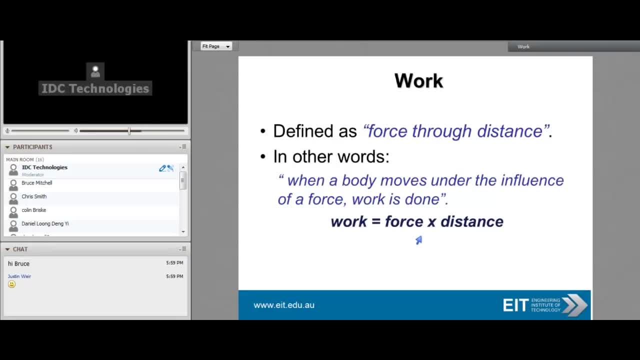 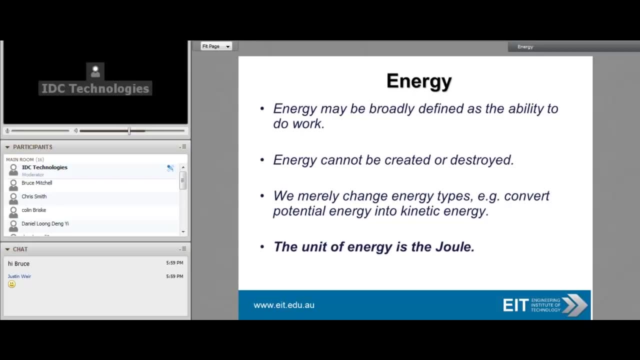 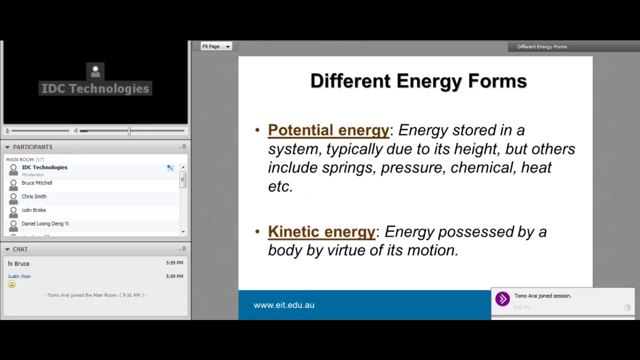 So we calculate work by multiplying force times the distance through which we move the object Energy. well, we know that energy can't be created or destroyed and the unit of energy is the joule, And there are basically two formats that energy can take a form in. 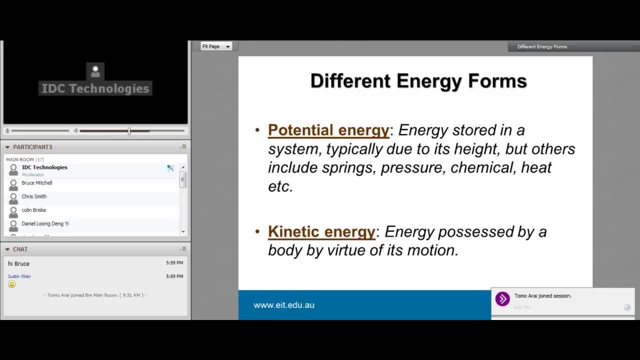 The first one is potential energy, That's the energy stored in springs, for example, the energy that a body has due to its height. If you think about a tank, a water tank suspended above a tank, it's a water tank. 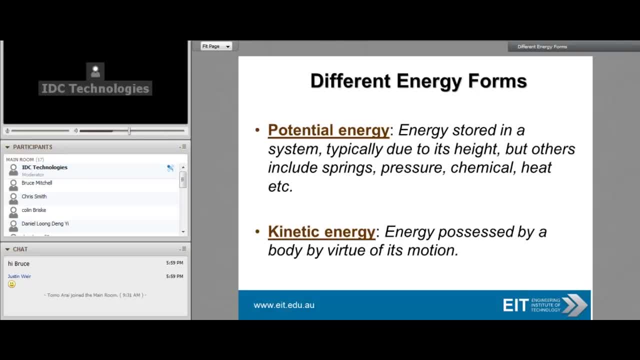 The higher that tank is suspended above the top, the more water will come out. as the top is opened, the more pressure we'll have. Kinetic energy- well, it comes from the Greek kini, meaning motion. Kinetic energy is the energy possessed by a body by virtue of its motion. 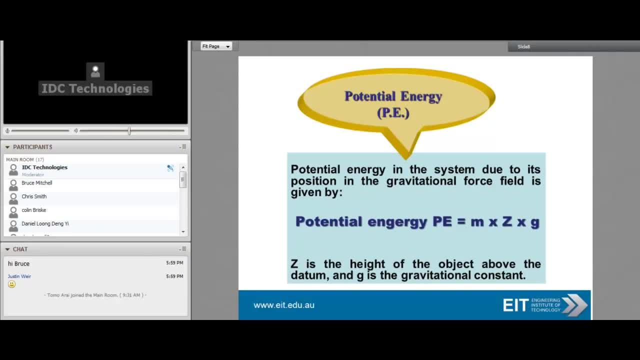 And these are basic things that we're going through now, guys. We've got to become familiar with them because we will be using them later. Potential energy: we can calculate that by taking the mass of the object multiplying the distance between the object and some datum that we set, multiplied by g, the gravitational. 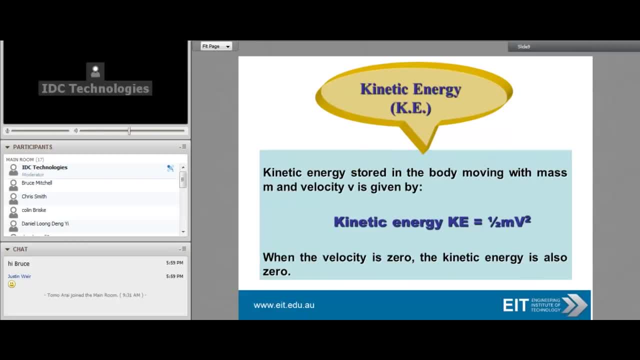 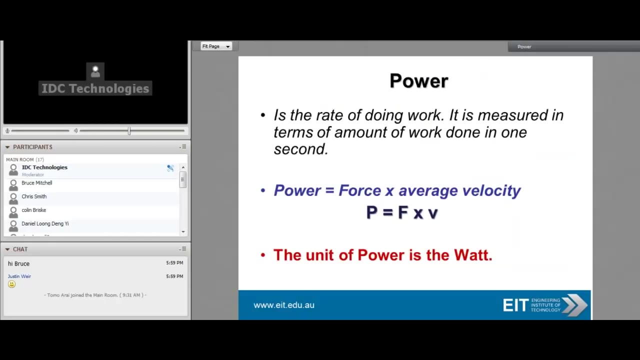 constant Kinetic energy. well, we can calculate that by taking half times the mass of the object times its velocity squared, And the velocity will be in liters per second. OK, now we're getting to some useful stuff now. Power. 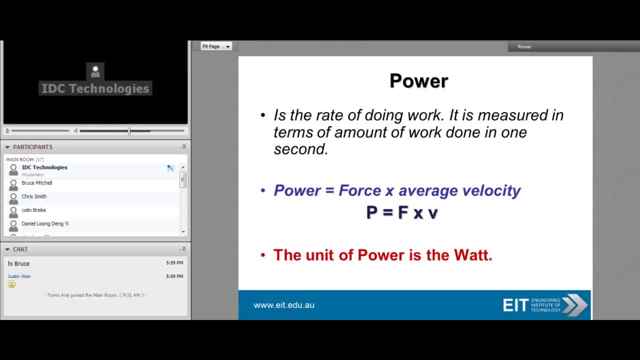 Well, power is the rate of doing work, And the way we can calculate power is by measuring the force multiplied by its average velocity, And the unit of power is the watt. What does thiseps 1060,000.. That's 8.2.. 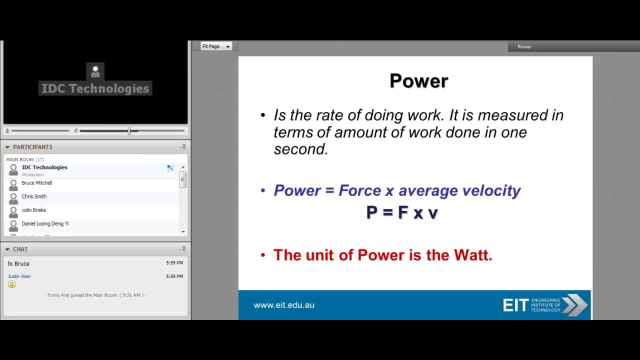 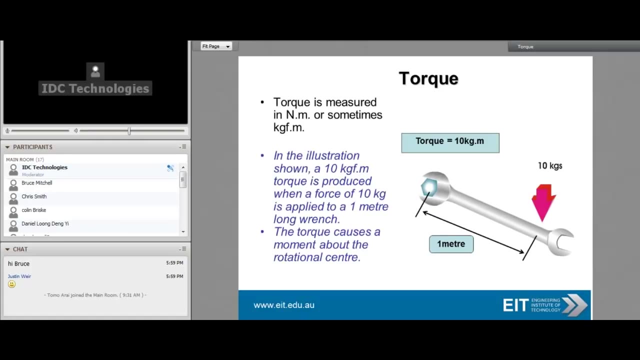 460.000. El sobre 10.. Unless you're in electronics, normally the machinery that we're utilizing for driving pumps and compressors, for example, or conveyors, is measured in kilowatts. Now, torque is basically force times. radius of application. 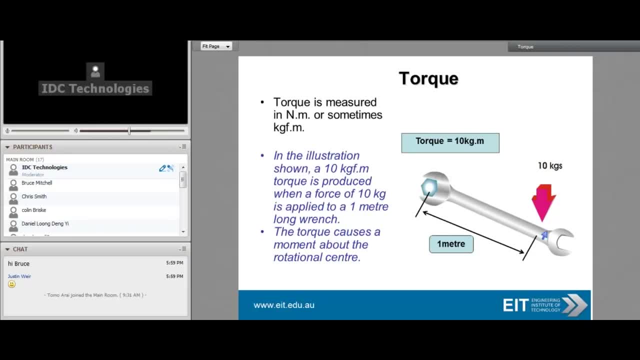 So you can see, here we've got a 10-kilogram force on a spanner and we're applying that force at a distance of one meter from the center of this bolt here. So we get a torque of 10-kilogram force meters. 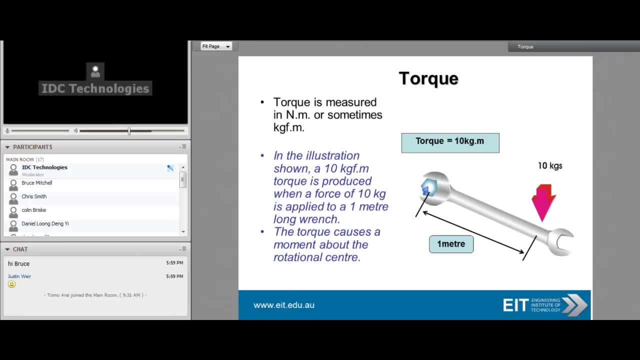 So the further away this force is applied, the more torque we get. The higher this force becomes here, Over a given distance, the more torque we get. So torque is a product of force: times, distance of application from, in this case, the center of the bolt. 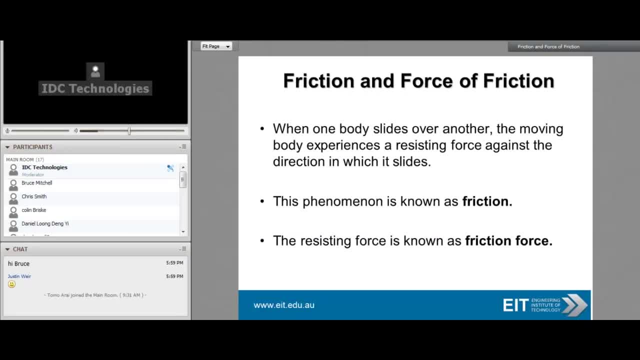 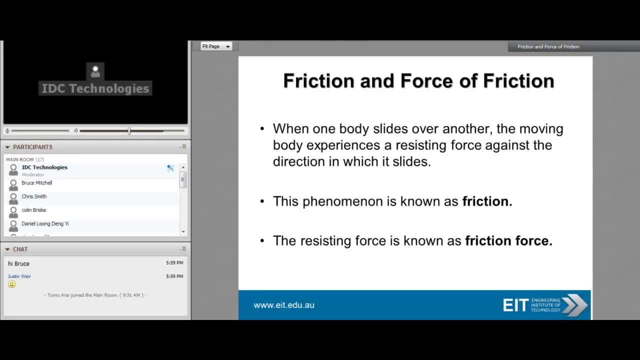 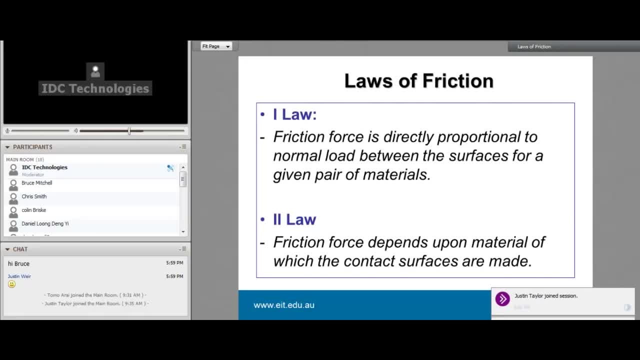 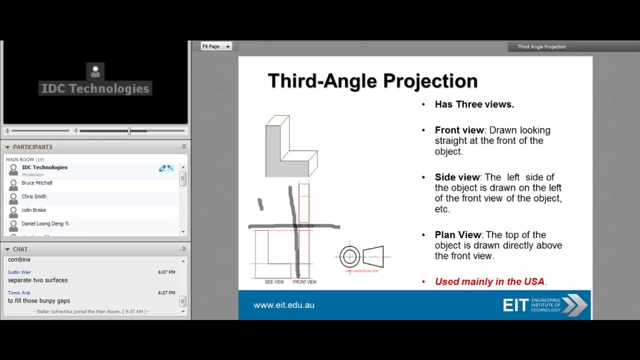 So if we have really rough surfaces, then we will have a high friction force between them when we try to move them. So if we have really rough surfaces, then we will have a high friction force between them when we try to move them. sorry, This is the first, this is the second, this is the third and this is the fourth. 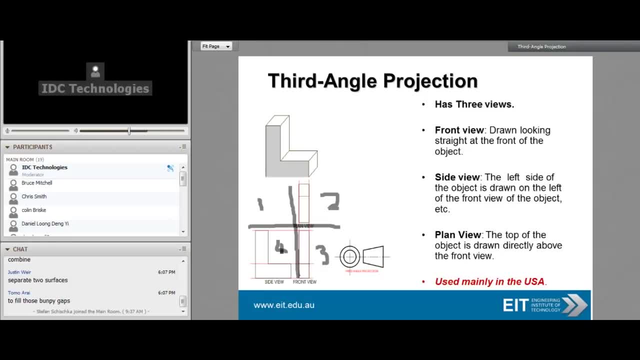 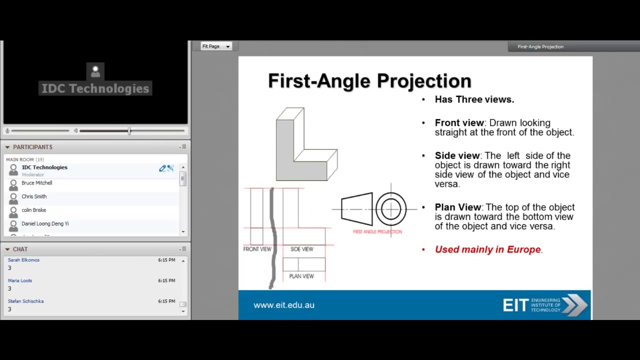 Now, where is the front view in third angle projection? Where is the front view in third angle projection? In which quadrant is it? Okay, everybody passed that tough question. Now let's look at first angle projection. Let's divide this into four again. Here's: 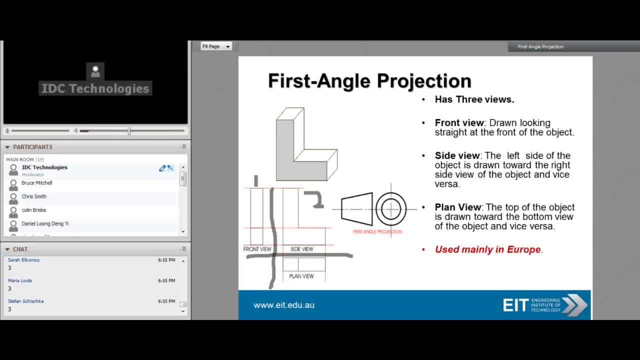 my first quadrant, second quadrant, third quadrant and fourth quadrant. Where is my front view now? Which quadrant is it in First? So that's a little trick I use, guys. You know everybody has their own methodology for these sort of things. That's how I. 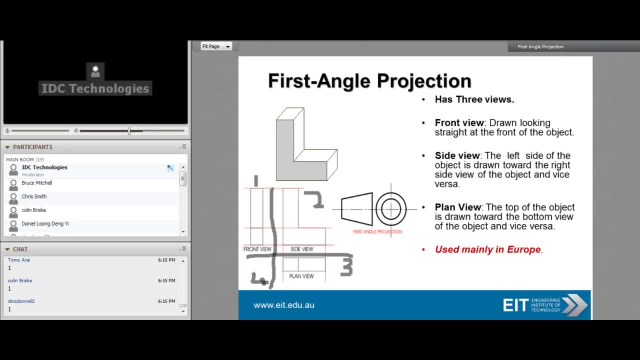 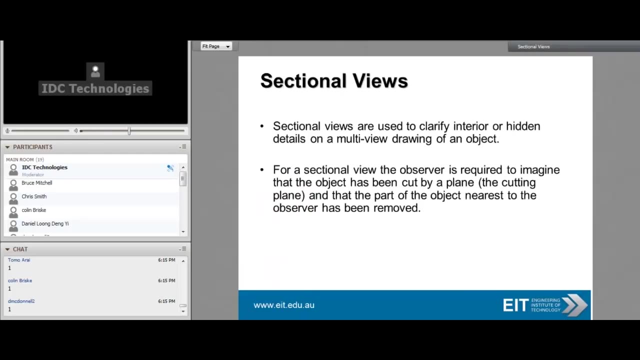 remember, when I'm looking at a drawing, whether you know, I don't have to look at the name or where it was printed in order to ascertain what type of projection it is. Now, I hope you'll find that useful to you. Moving on Sectional views are very, very useful. They're. 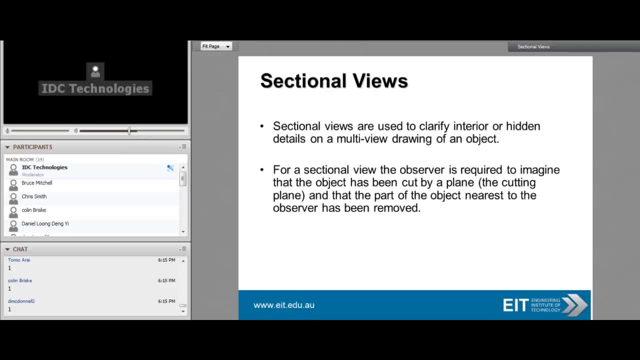 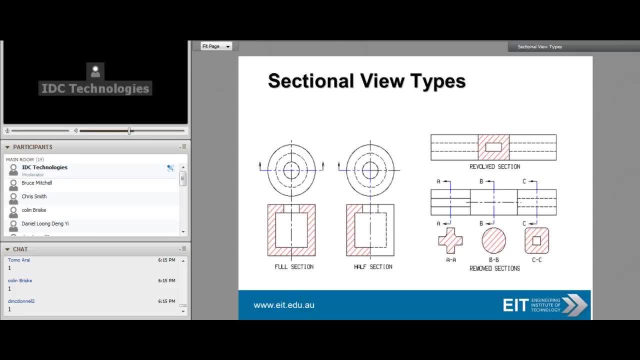 so powerful guys. They really help you understand what's going on. what you're looking at when you look at a drawing And a sectional view is an imaginary slice through an object so that you can see what it looks like. Now, here in the top view, here, what we're looking at is we're looking 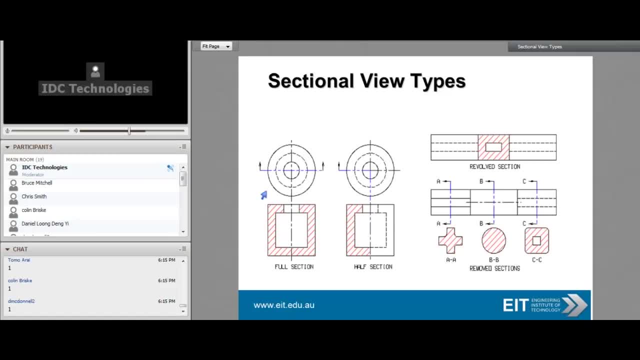 at what looks like a cylinder with a hole drilled in the middle and some kind of hidden object here. But look, if we didn't have a sectional drawing, we'd think that it's going to be a hole in the middle. And the answer is yes, it's not. But if we had a sectional 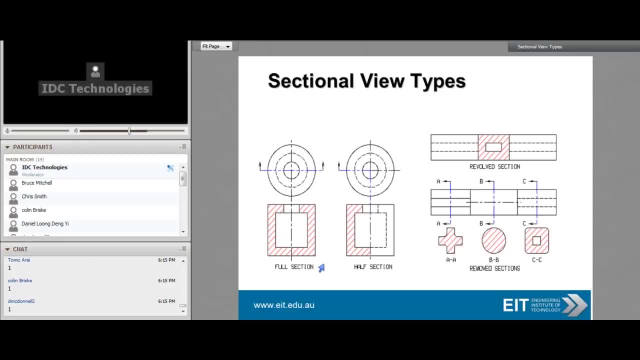 view, we would say that that hole went right through, wouldn't we? And the natural fact it doesn't. This full-section view and these lines here are called cross-hatching. This full-section view shows us that that hole is only in the top half of this object. It 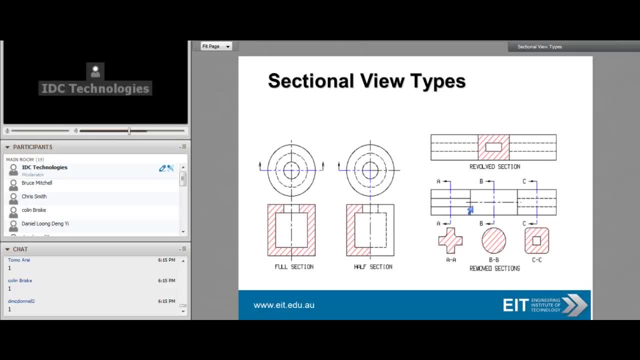 doesn't actually go all the way through, And here is a half section which we sometimes use. Now let's take a look at this one here on the right. This is mind-blowing. Look at this view here: This is the top half of an object. Look here, This is the top half of an object. 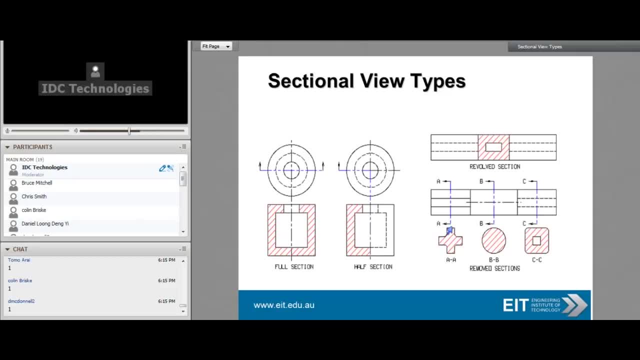 Just look at that, You'll notice that there's a whole section of the object, And this is the view here. So what we have is in this part, the first part of the object, here we've got two solid lines. Now that could be a groove or it could be a raised portion, like it's. 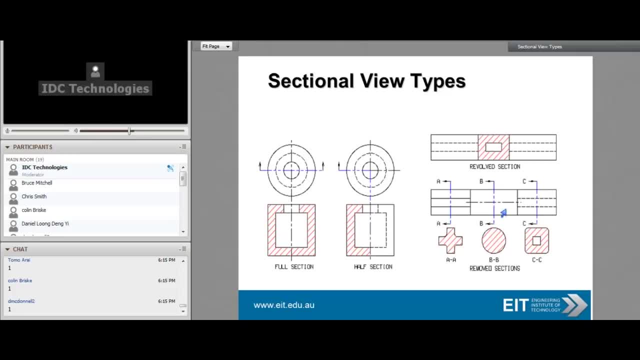 shown here. Then we've got a center line here. What do you think this could be? What section do you think this could be? Just looking at this drawing here, what type of section do you think that could be? There's two lines there. 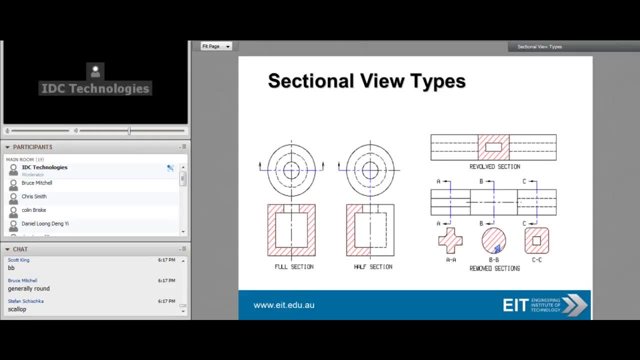 What could they represent? Well, we see, one of these things is that, yeah, it's round, but what other section could it be? Stefan, it wouldn't be a scallop. I know what you're saying. It's just like a U-section. you wouldn't see a center line there. 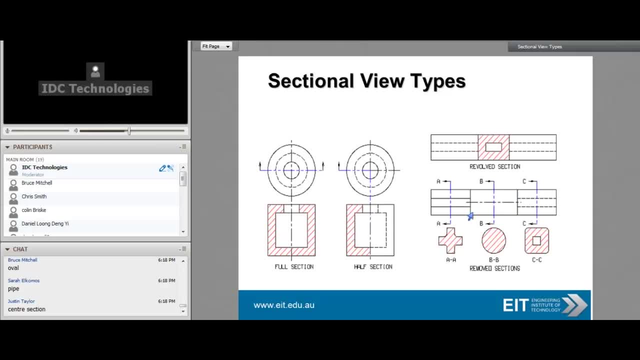 It could be an oval. Yes, it could be Good one. The other thing, what about it? It could be a rectangle, or it could be a square, couldn't it? What we're seeing is two lines here, or four lines here. 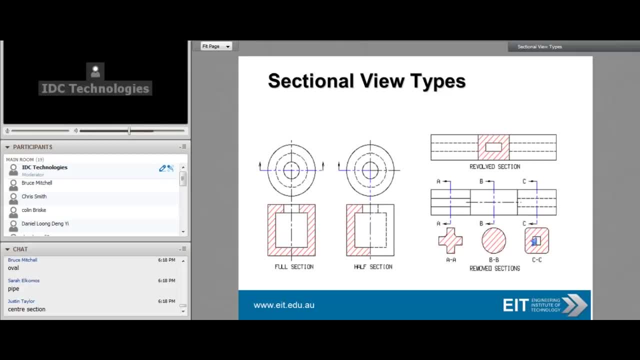 So by taking a cross-section, in this case here, BB BB shows us the section is actually round. How about this guy here? It shows you a square hole in there. What else could this be here, represented by two dotted lines here. 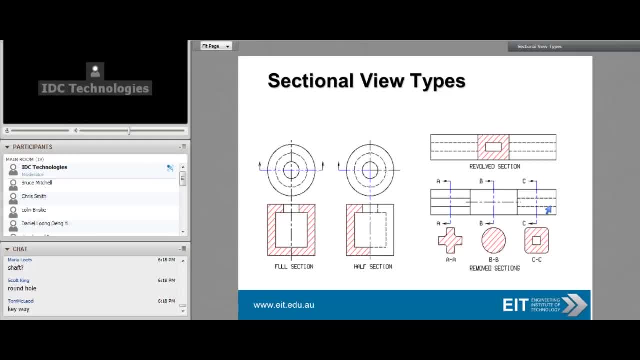 What else could that be? It shows here in the section it's actually square. but what else could it be here? Well, it could be a round hole, couldn't it? It could be drilled. Yes, It could be round. Here it's shown square in actual fact. 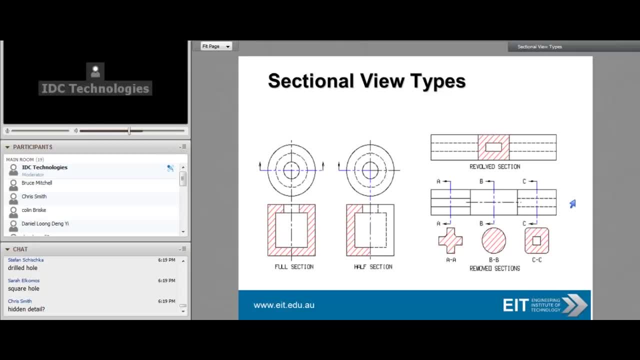 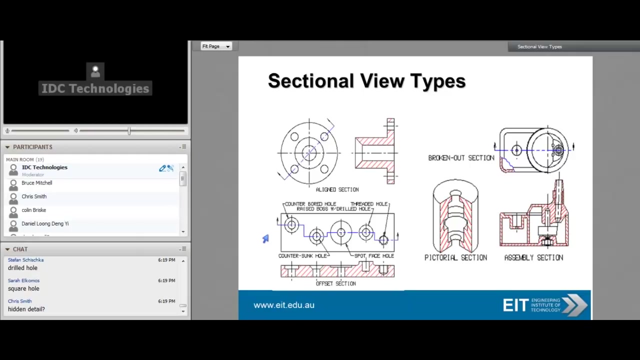 So can you see how this is all hidden detail here? It's all hidden detail, but how, using sectional views, how a lot more information is revealed, And that's why these are very powerful details on a drawing, very useful to someone that's got to manufacture this. 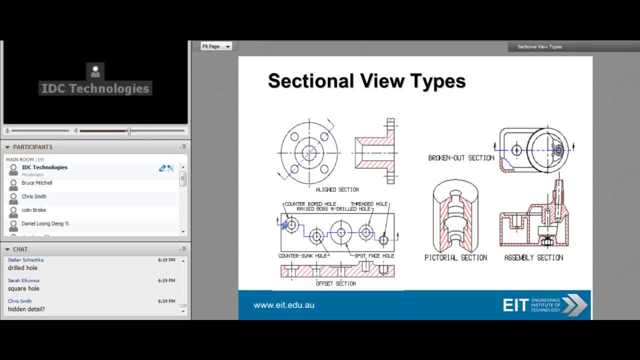 How about these sectional views? Let's take a look at this plate here. Wow, Well, this is countersunk, but is it a square countersunk or is it a taper countersunk? Because look at this hole here on the right and look at that hole there on the right. 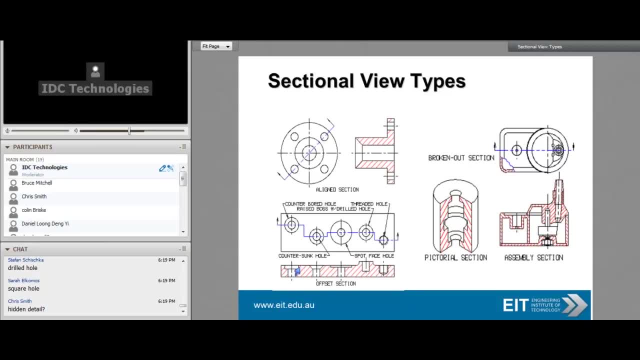 They look exactly the same in this view, don't they? But now take a look in the cross-section. We can see this is actually countersunk square, countersunk tapered. How about this one This? obviously it's shown in dotted lines. 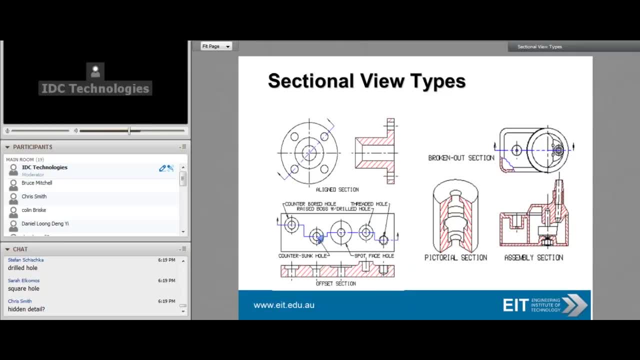 That would go actually three-quarters of the way around there to represent a tapped hole. Look at this. That looks the same as that and the same as that, doesn't it? But in this case it's actually a raised face here. 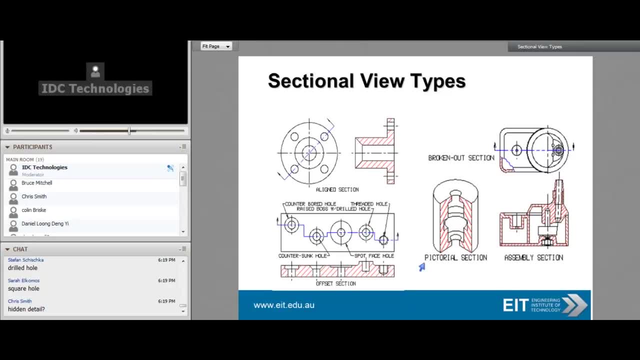 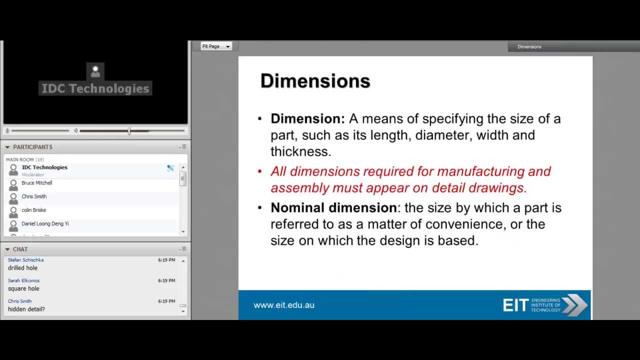 It's a raised section that's been spot-faced, It's been machined and it's round. It happens to be round. So wow, Do we need to explain any more about how powerful sectional views are? They do reveal a lot of information, don't they? 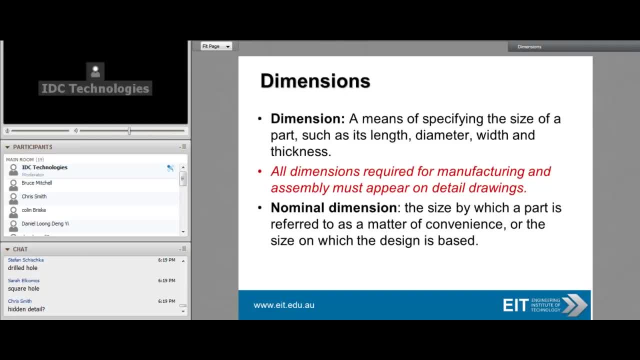 Let's talk about dimensions. Well, why do we need dimensions? Why do we need dimensions, guys? Why do we need dimensions? Now, don't give me any of these answers here, because it's all in front of me as well as in front of you. 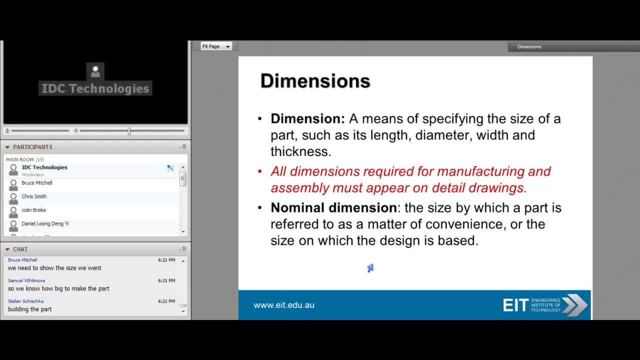 But what other reason do you think, Apart from what's here on the slide? do we need dimensions on a drawing? Well, yes, we've got some pretty good answers there, Folks. the answer that I was looking for is: if you have drawings on a sorry, a drawing with dimensions on. 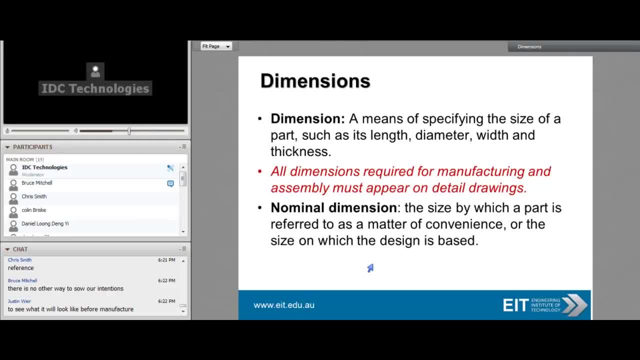 we said that the purpose of drawings are to communicate between the draftsman and the operator, the machinist. Now the operator, the machinist, makes the part according to the drawing. How do we know it's right? How do you? how do we know? how do we know the machinist has made the part correctly? 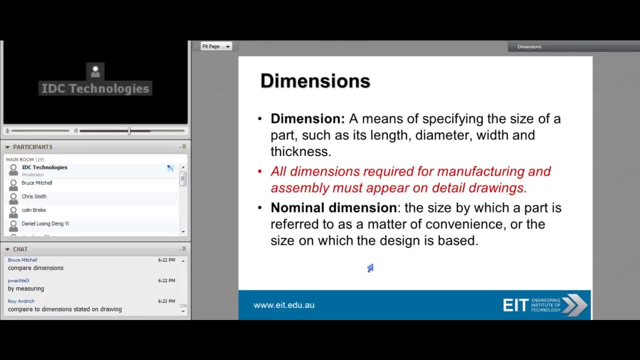 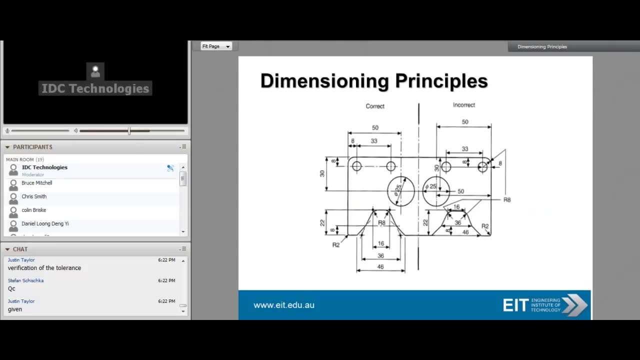 Yes, Scott, On the money Bullseye. Yes, Bruce, Yes, Roy. We compare the dimensions that we measure On the money, On the actual manufactured part, against those stated in the drawings. Now just a word about drawings here before we start talking about limits and tolerances, because I'm just bringing us into the next subject a little bit prematurely. 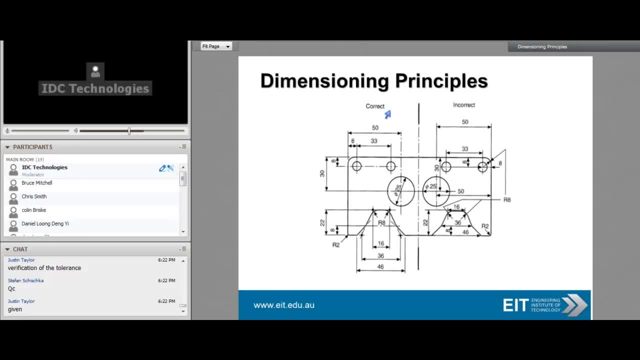 Take a look at this drawing. Can anybody tell me why we would say this part here? imagine this: we've got two drawings mirror image of each other. This part here There's a mirror image of that part. Take a look at the way that they're dimensioned. 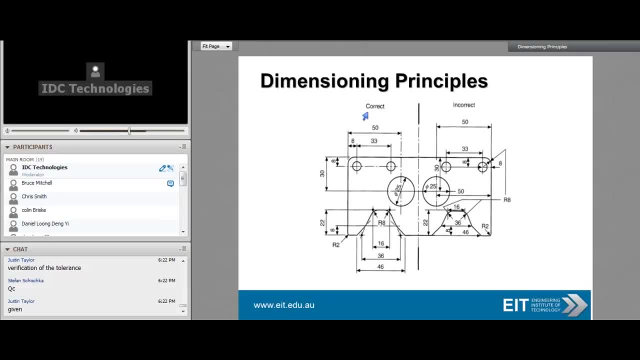 What strikes you as being the reason we've labeled this side, the left-hand side drawing, to be correct and this one incorrect. We've got all the dimensions that we need here, on this part here, This part here on the right, all the dimensions that we need on the left. 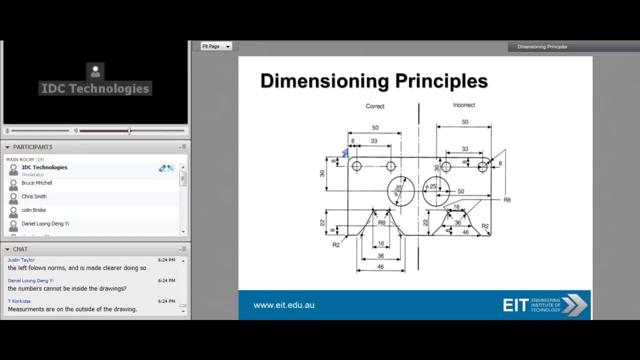 But why would we say that this drawing dimensioned here is correct and this one is incorrect? Well, I'll give you a little bit. Well, yeah, the first thing that strikes you is the dimensioning here on the right is nowhere near as clear as the dimensioning on the left. 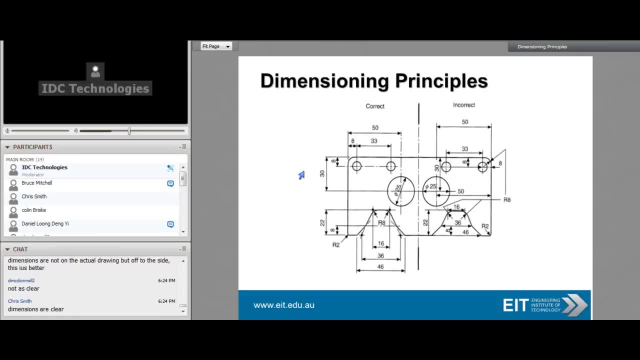 It's a lot neater. Also, we're working from a datum. If you're a machinist, I need to know how far away from this side here to put this hole in and that hole in there and then this hole in here. 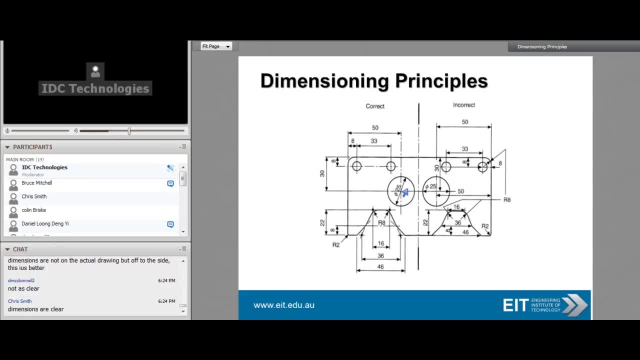 So it's very easy. I don't have to add up the dimensions in this drawing, But you guys got it right. You said we are aware that the reason that this is correct is because the drawing is a lot tidier. It's a lot easier to understand. 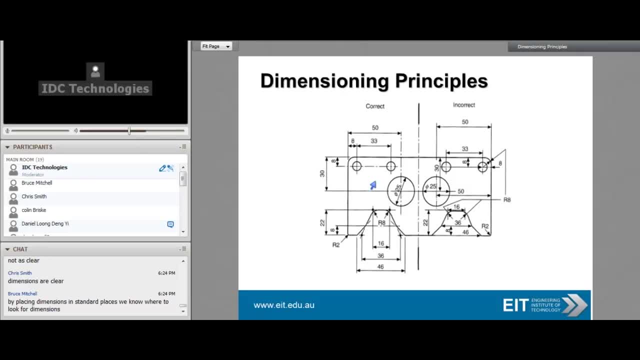 We don't have any dimensions that are actually on the drawing. They're away from the drawing so we can actually see the part much clearer. I mean, this is really confusing. What do you think would happen if we sent this down to the machine shop for the machinist? 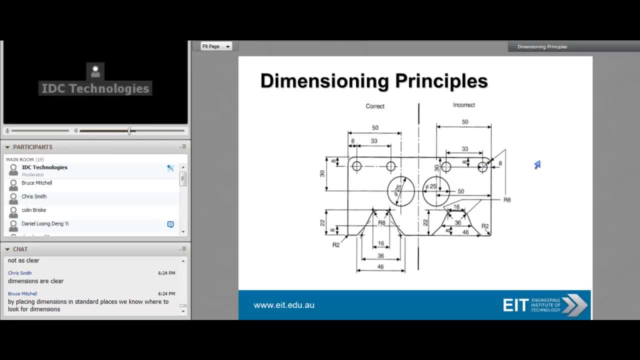 to manufacture. What do you think might happen there? Absolutely people, 100% correct. Well, yeah, If I was the machinist, I wouldn't be impressed by the drawing either. You should. Good answer, But there's always a much greater risk. 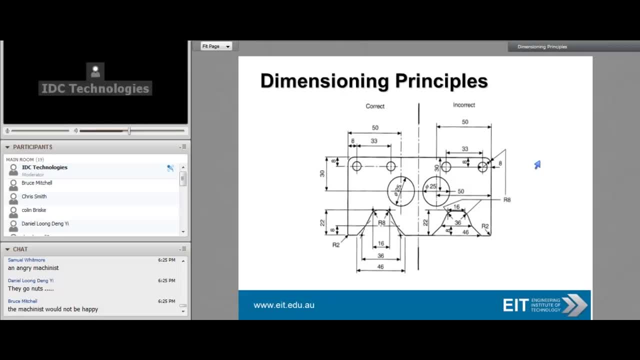 Much greater risk of producing the wrong article. The machinist would have to sit there and try and work through this maze of dimensions as to how to produce this article. And yes, Justin, yeah, it takes time, And time, as we know, is money. 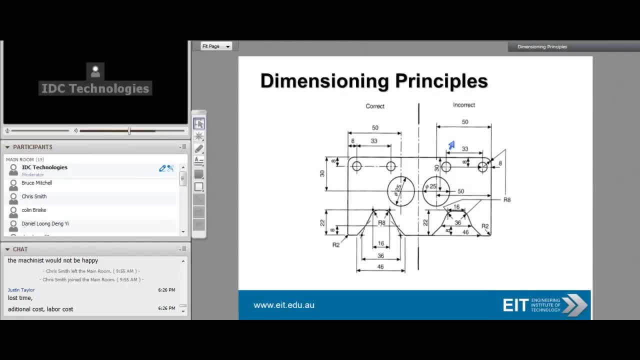 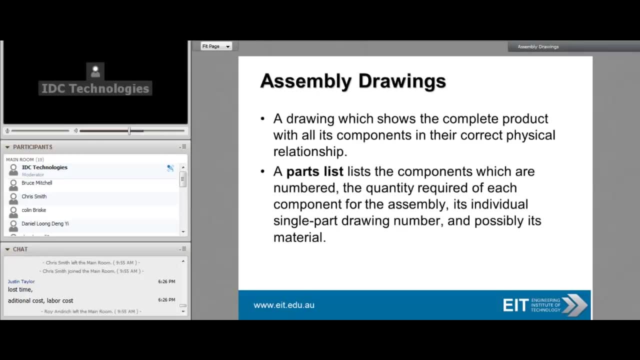 So yeah, Bigger chance here of producing scrap when compared to this dimensioned part of the drawing. Good one, Very good, Okay. Moving on, Another useful drawing for us, especially if we're going to put parts together, is an. 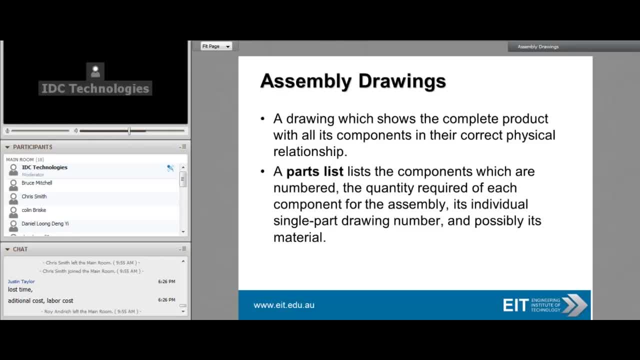 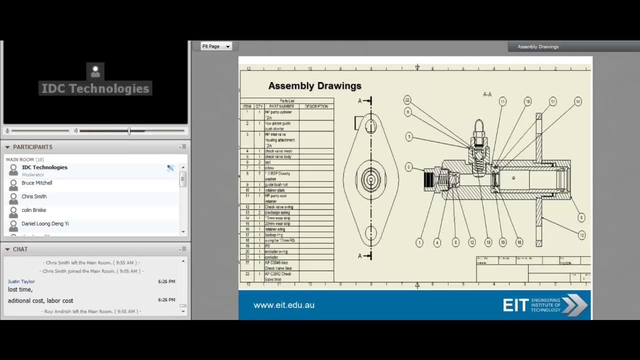 assembly drawing, And an assembly drawing shows how things are put together And generally one can assemble it. It's like a Lego set if we look at this Now. the assembly drawing, The assembly drawing, shows how things go together And we have a parts list along with the drawing. 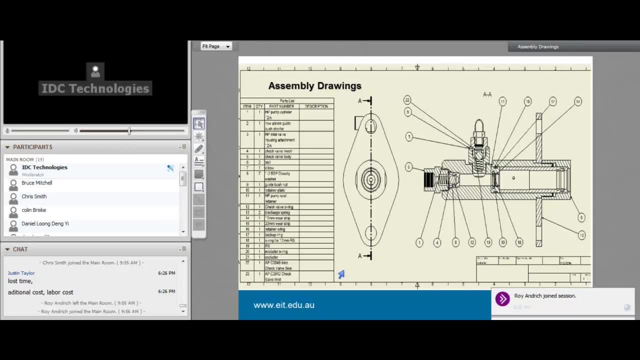 What do you think the parts list helps us to achieve? What purpose does the parts list serve? should I say Yes, Scott? Yes, It identifies the components Because- bear in mind people- this is an assembly drawing, but each individual part has to be. 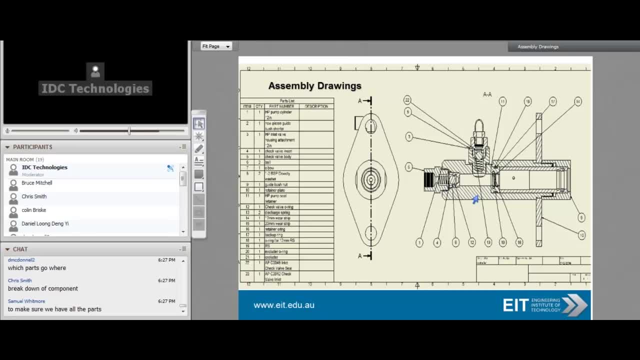 machined. So in this column here it says description. There's a part number. Actually that's the part description. really, to be strictly strict, This is the description. There should be a number in here, a machining drawing number in here, so that we can identify. 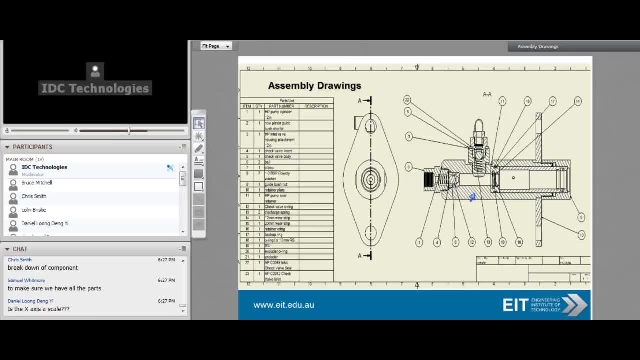 the component. Also, when you look at the parts list, it tells you how many of each part we need, And that's also useful, isn't it? The x-axis? no, Daniel, The x is a section. It's just to show that this drawing is a section view. 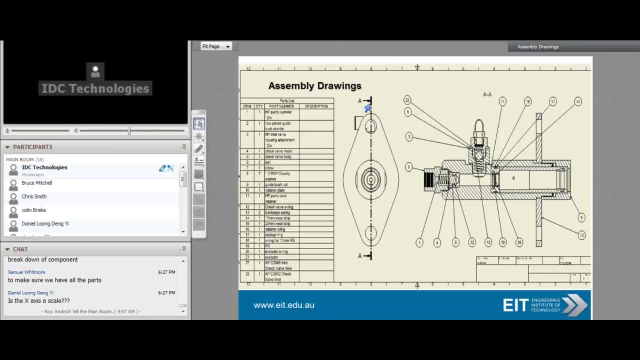 Viewing on AA. So, in other words, I take a hacksaw, I cut this imaginary hacksaw, I cut this in half, and what I'm seeing here on the right of the drawing, is the view that I would get if I looked at the component once it's cut in half from left to right. 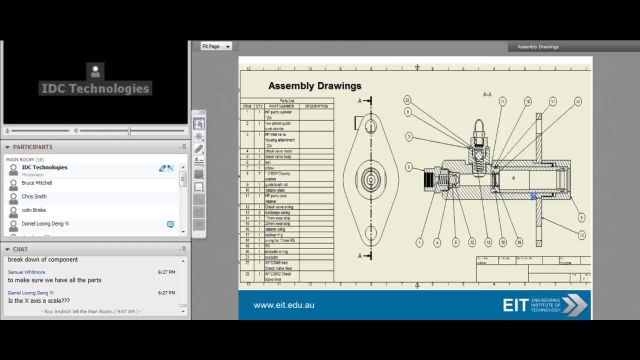 Any idea what this might be, guys, What this component might be? Yeah, it's a hydraulic piston. It's a hydraulic piston. I actually believe it's off a brake master cylinder. Oh, well done, Bruce. Yeah, I believe it's off a brake master cylinder. 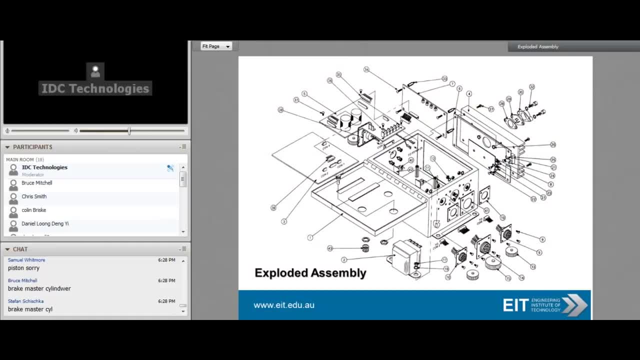 Well, that doesn't tell you that there. Well done. You guys are on the ball today. Wow, Look at this exploded assembly. I did say it shows us how things go together. I think this is pretty good in determining where we are, how things fit together, where. 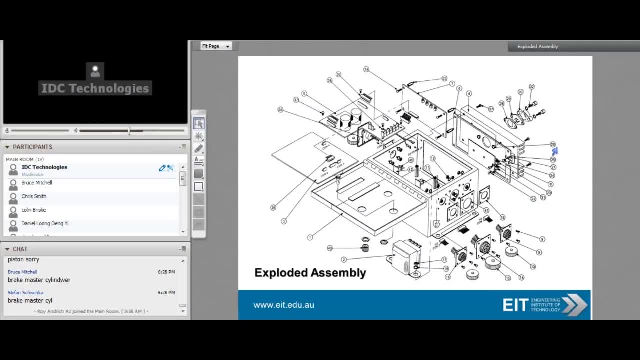 they should go and you'll notice we've also got item numbers on here. What is the purpose of those item numbers? Why do we have item numbers on an exploded assembly? Yeah, Okay, Yep, You guys are definitely awake. It's to identify the parts and to go back and look at them so we can go back refer. 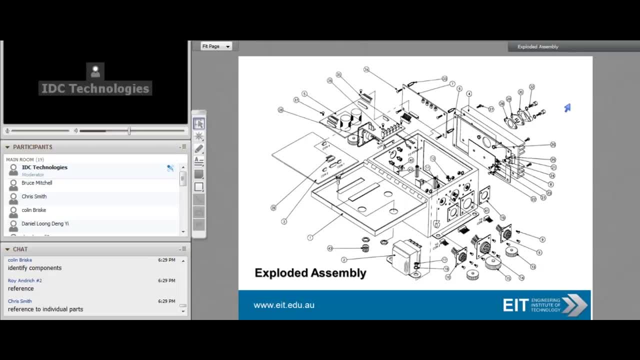 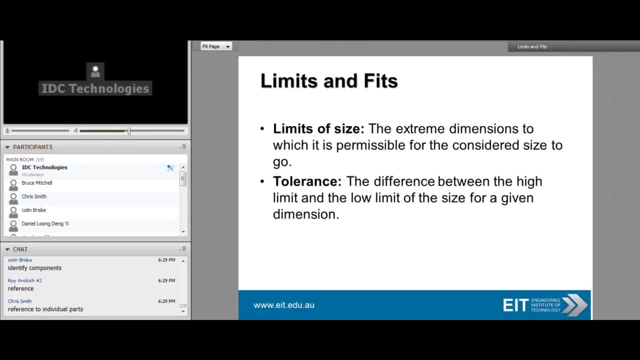 to the actual manufacturing drawing. Good Now, before we talked about, you know, dimensioning things and manufacturing things and hopefully we'd get them right Now. we're going to talk a little bit now about limits and fits, And the limits of size are the extreme dimensions, the maximum size. the minimum size which? 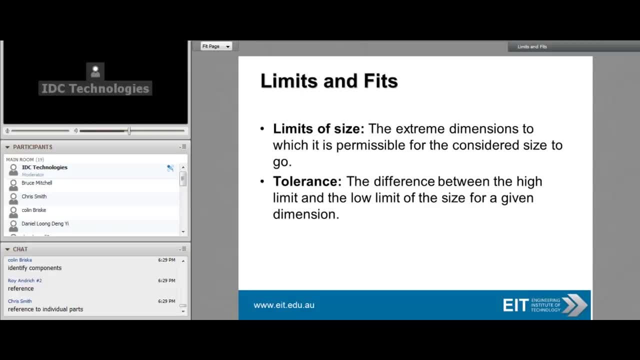 is permissible for a component to be made. Now designers often calculate and design a shaft to fit in their hole. Now the cost of the manufacturing of this depends on the limits that we apply to the shaft and to the hole. If we make the dimensions of the shaft extremely tight, in other words, we allow very, very 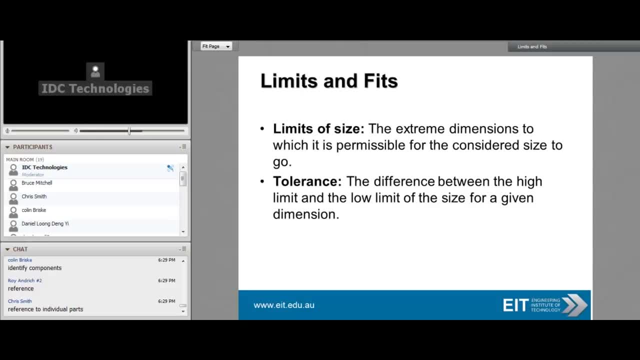 very little for manufacturing errors, then that shaft will be expensive to manufacture And often the designers decide what the final dimensions should be for mating parts. Now, limits are normally used for cylindrical holes and shafts, but they can be used on any part, or parts, rather, that fit together, regardless of what they look like. 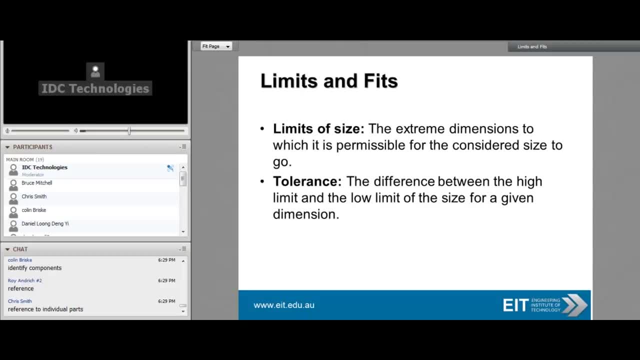 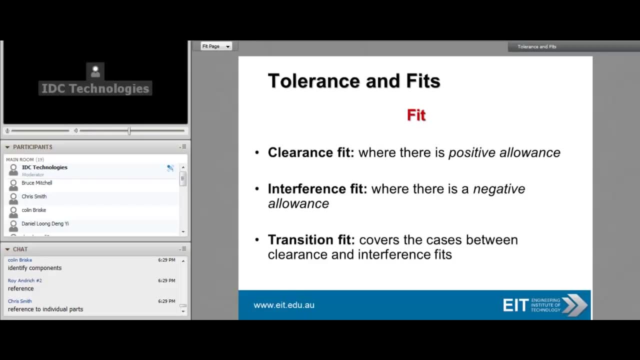 Now typically a limit is the upper and lower tolerance for a shaft or hole. Now we've got different types of fit between components. We can have a clearance limit, We can have a clearance limit. We can have a clearance fit where a pump shaft fits into a plain bearing and that shaft 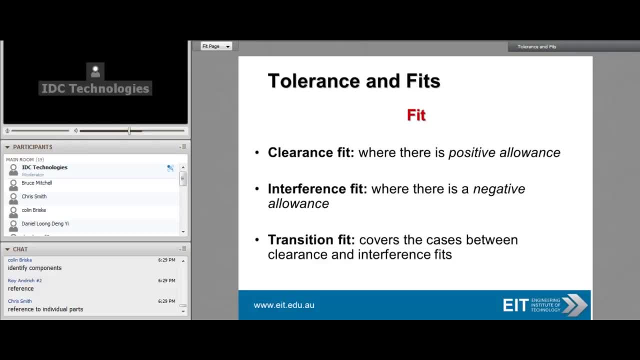 rotates in the bearing, hopefully with some kind of lubrication there, and that is a clearance fit. An interference fit is where there's a negative allowance. You may want to put two halves of a tool together with a dowel, and the dowel size is slightly. 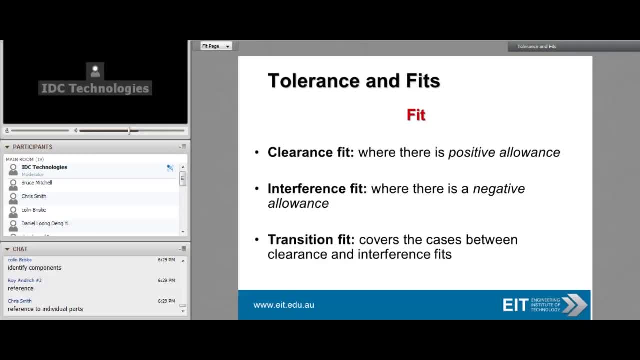 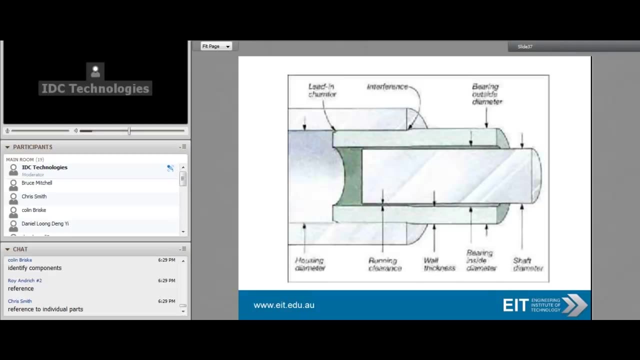 larger than the hole size in one half of the tool, And then we've got something that's in between a clearance fit and an interference fit. It's called a transitional fit. Let's take a look at an example here. So we're looking at a drawing of a housing, a bearing bush and a shaft here. 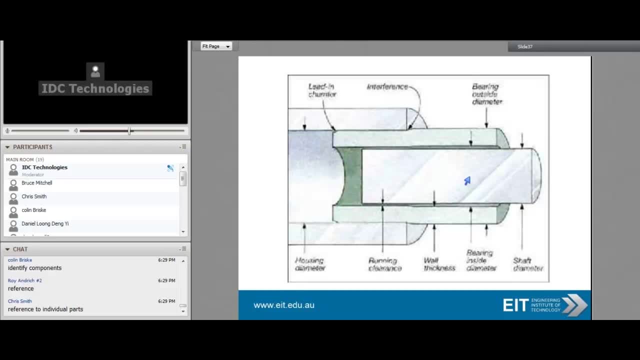 What type of fit do you think that there is between the bearing bush and the housing? So this shaft will rotate in this bearing bush and this is fitted inside the housing. Well, yes, it's an interference fit. It's pressed. The bush would be pressed into the housing so that it doesn't rotate. 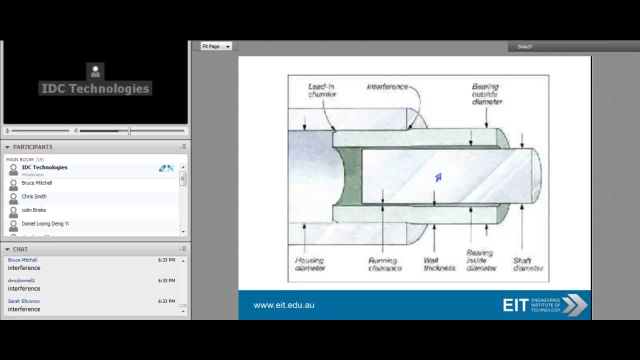 Now let's look at the shaft. We've got the shaft rotating in this bearing bush here. Now ignore the drawing. What type of fit would you think that the shaft is in the bearing bush? Oh, some of you. you got it already. 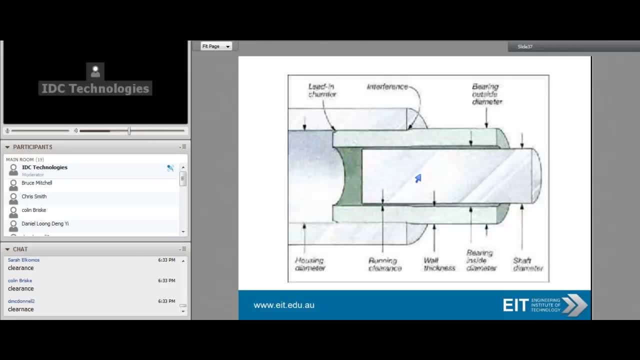 You got it. Well done, guys. It's a clearance fit. It's a clearance fit. So what we would do in this case of this assembly is we would put nominal sizes for the shaft, the bearing bush and the housing and put tolerances on to ensure that we get the correct fit. 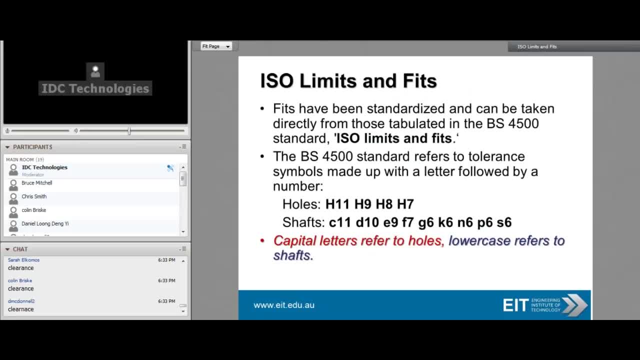 And our designers refer to iron, They refer to straight and square And they say: well, if you have a good fit, you can put it on a lot of things. So the steel is a little bit more than just a little bit of a little bit, and it's a 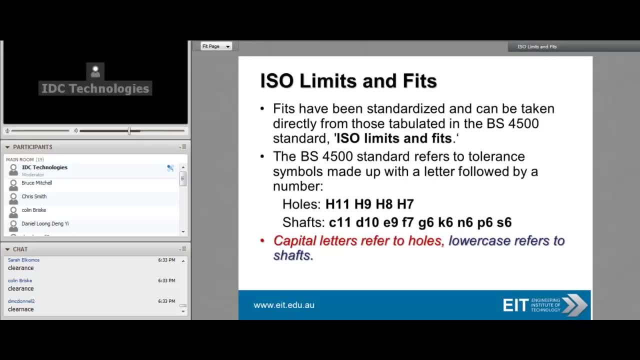 little bit more than just a little bit, and it's a little bit more than just a little bit. So there are a few things that we can do with this. The first is we can use a standard of 4500.. And there is a standard which is British standards 4500,, which is an abbreviated table. 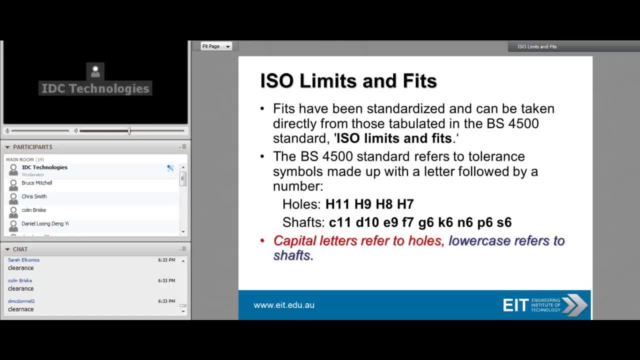 if you like, And you'll see the table in a moment and you'll understand immediately why we use letters. It's a shorthand, basically, on a drawing. Now, all we have to know for the sake of this webinar is that holes are specific for the. 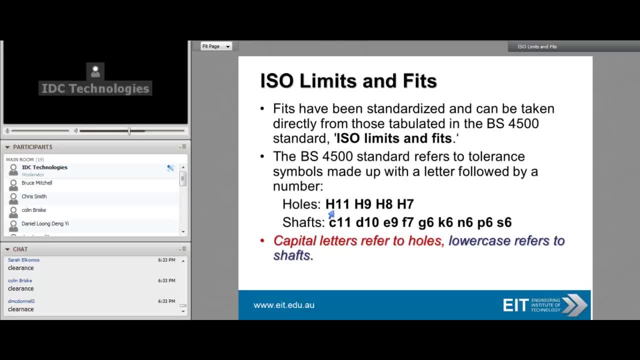 are designated by a capital letter and shafts are designated by a lower case. So we've got H11, H9,, H8, H7, which refers to holes, and then we've got C11, D, 10, E9, etc. etc. 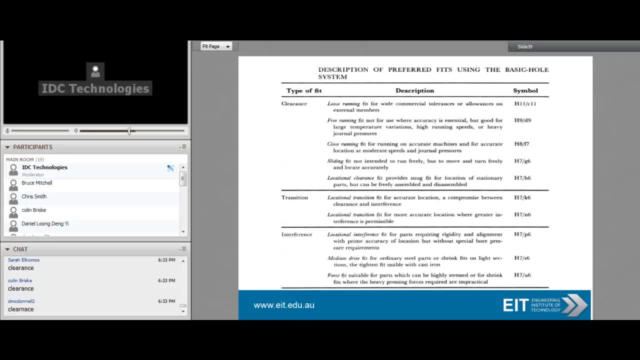 which refers to shafts. And here's the table. here, guys, Now can you imagine producing a drawing and then having to write free running fit, not for use where accuracy is essential, but good for large temperature variations. high running speeds are heavy. 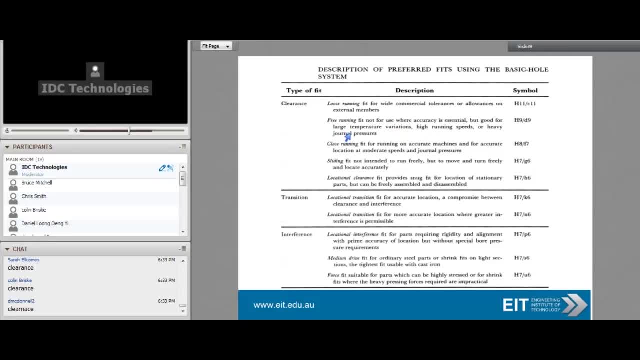 to pull up. I'm getting tired just saying it. Imagine having to put all of this text on a drawing when you can just do this: H9, D9.. Which would you prefer to do? Write all of this out or put this in your on your drawing? I think I know what the answer is. 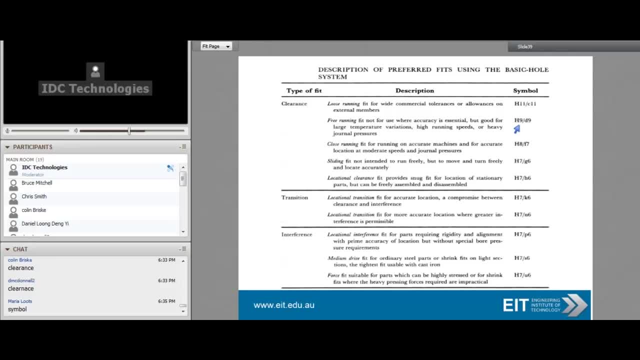 going to be. It's going to be before I even see your reply to that one. So under clearance fits we have all of these symbols that one would refer to, and these go from loose running to location clearance, And all of these are defined by the large. 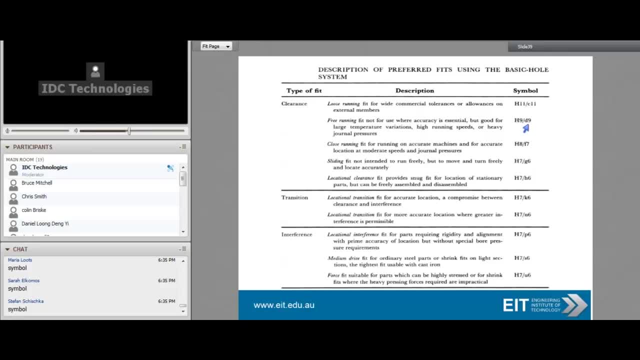 letter H and a lower case letter here, in this case D Transition. Then we've got different types of transition. There's the locational transition fit for accurate location And it's a compromise between clearance That's a rattling fit and an interference fit where 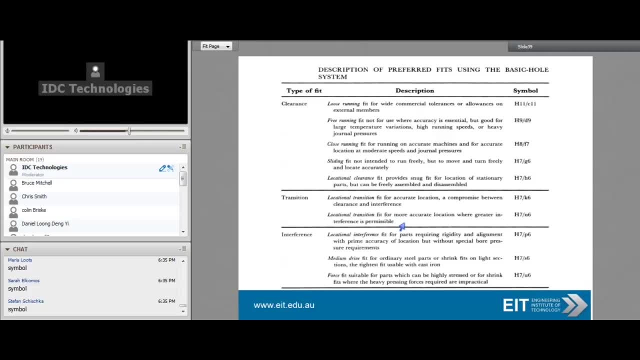 it really has to be pressed in. And then we've got location trans transition fit for more accurate location where we've got very, very little clearance, And we then have that positional transition fit- which clearance at all? and we're having to make sure that the parts that are fitting together. 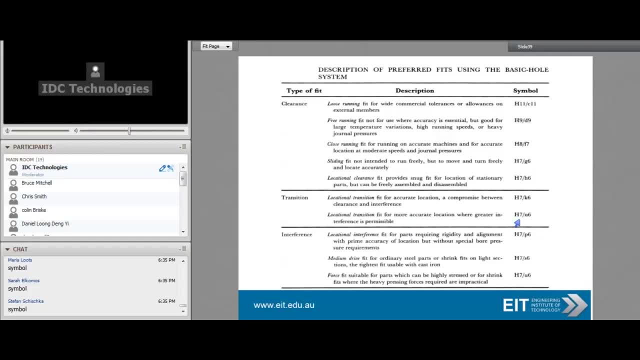 don't move, And you see the difference. here We've got H7.. What is the large letter designate? It's checking that you're awake. So in both cases we've got an H7, and in the first case we've got a K6, and in the second case we've got an N6.. So all this is, guys, is an abbreviated. 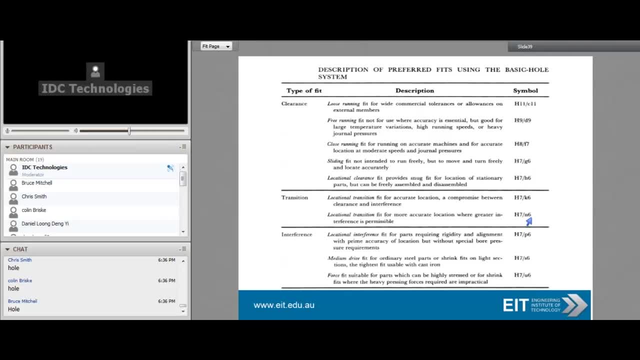 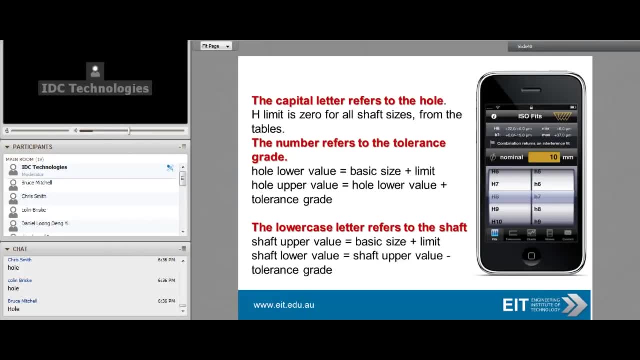 way of saying this to the machinist and everybody that's reading the drawing. And here we've got an example. here There's a little calculator that shows us that we've got an H7 and an H8. So we've got an H7 and an H8. And here we've got an example. here There's a little. calculator that shows us that we've got an H7 and an H8. And here we've got an H7 and an H8. And here we've got an H7 and an H8. And here we've got an H7 and an H8. And our nominal: 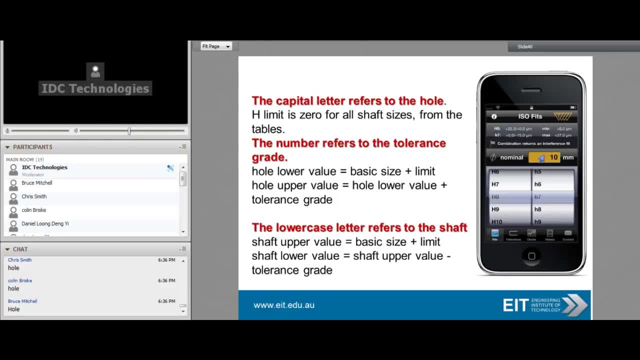 shaft size is 10 millimeters And we can see here the tolerance we've got here. H8, which is your hull size, can be 10 millimeters plus 22 microns and not any smaller. So it can be 10 millimeters plus 22 microns plus nothing. So it's either 10 millimeters or 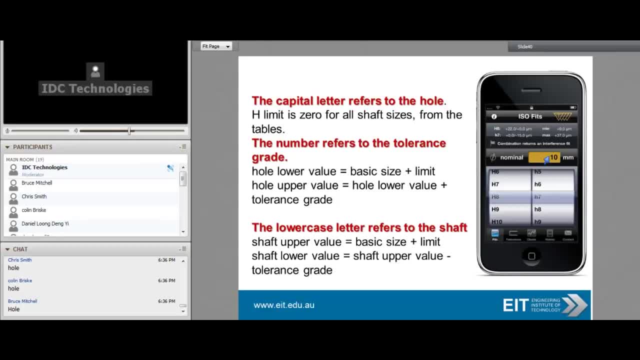 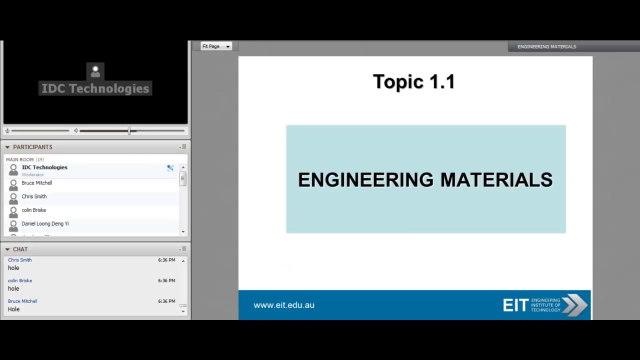 or 10.0 to 2 millimeters. That's your hole, And similarly for the shaft. the shaft is not going to be any bigger than 10 millimeters, but it can be 10 millimeters minus 0, minus 15.. And that's why, or how, we tolerance things in order to get the desired fit. 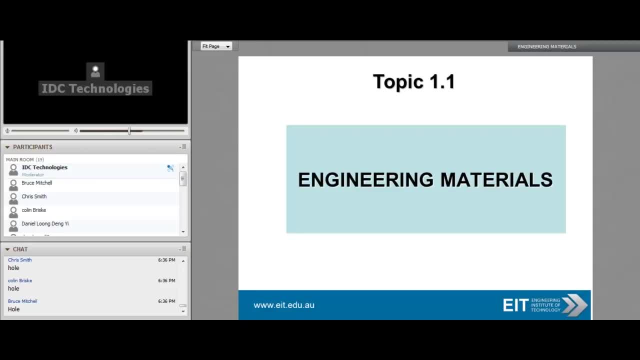 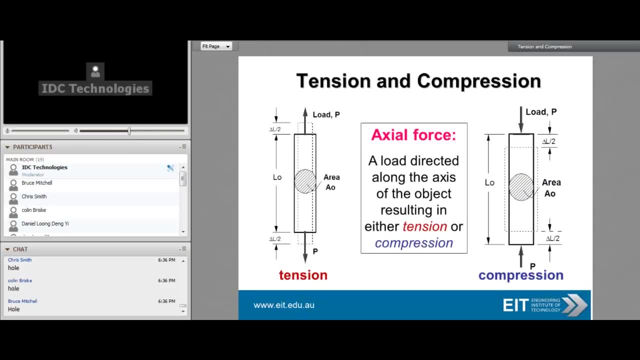 All right, Moving on, Let's now discuss engineering materials, And this is important, guys. Engineers need to know how materials behave under different conditions. Now let's get something out of the way. The difference between tension and compression is if you compress something. 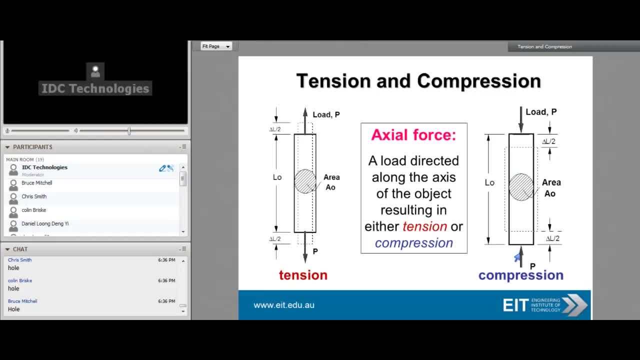 you press, You push it together. These loads are pushing together In tension. we're pulling apart. We're pulling apart. So, if a spring is being compressed, is it going to get larger or smaller? It's dimensions, It's length? If a spring is being compressed, will it get smaller or larger? 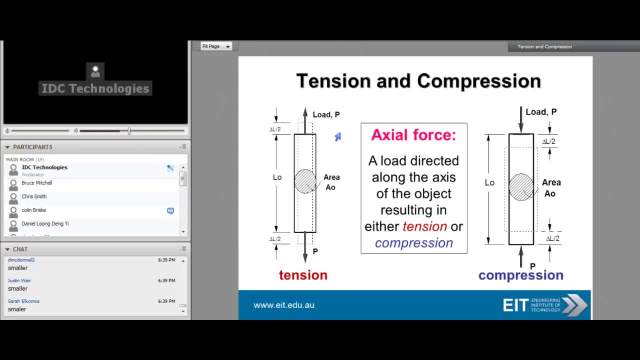 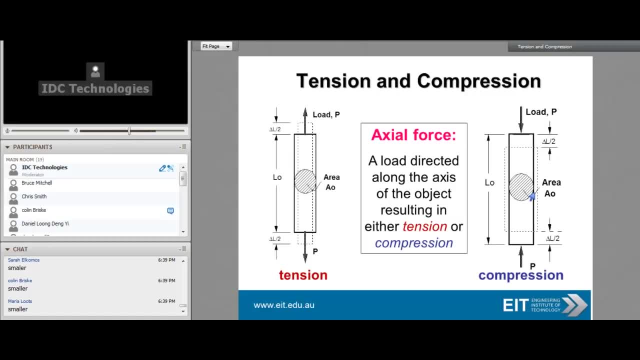 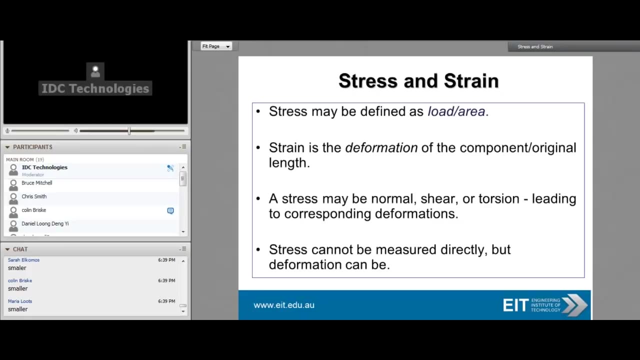 is applied to a rod of cross-sectional area A0. And in this case we've got a load that's pulling these apart, That's in tension. So both of those rods would be under stress. One would be being compressed, The other one would be being stretched, And the stress in both cases would be the load that we apply. 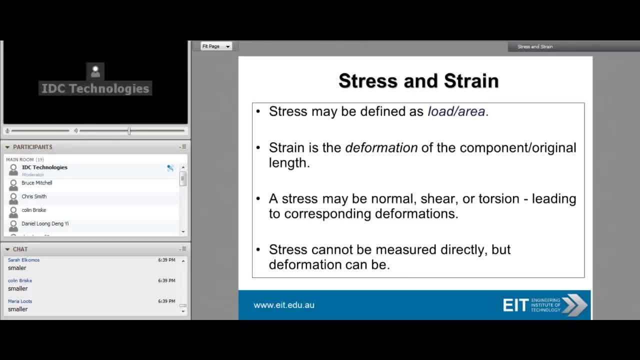 divided by the cross-sectional area. Strain is the deformation of the component divided by its original length. Now, stresses can be shear stresses, where we're trying to chop something in half, or they can be torsional stresses, where we're trying to twist something, or it can be a. 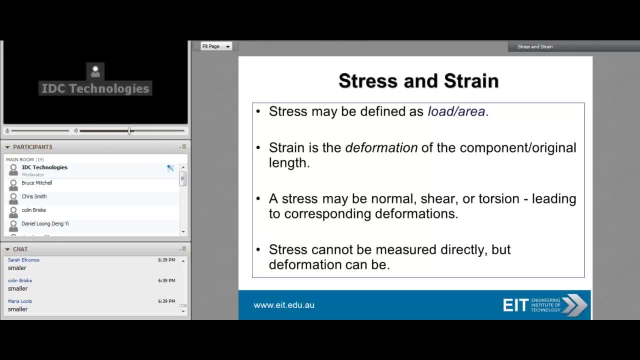 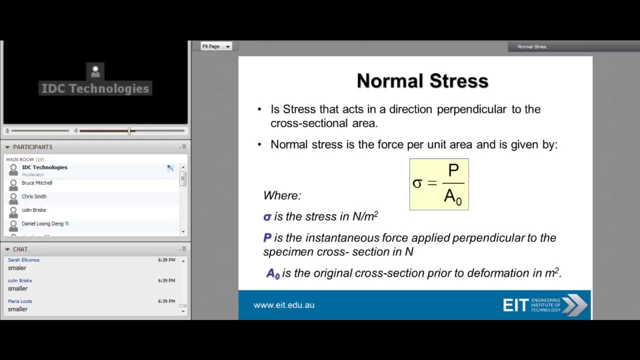 tensile stress or a compressive stress, as we saw before. Now we can't measure stress itself, but we can measure deformation, We can measure the change in cross-section. So if we talk about normal stress, normal stress is the force per unit area, that's. 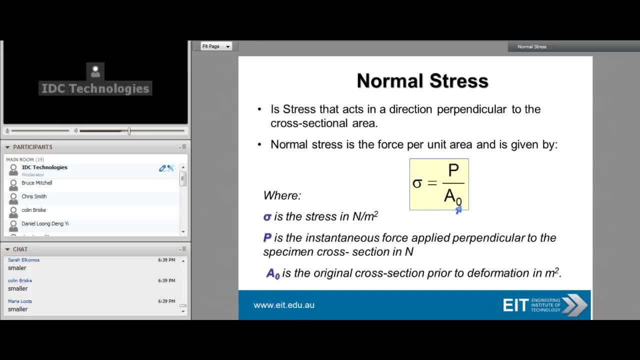 P divided by the cross-sectional area, A, naught And sigma is the stress in newtons per square meter. so P must be in newtons and area must be in square meters. Wow, tough maths, tough maths. Now let's go to an example. 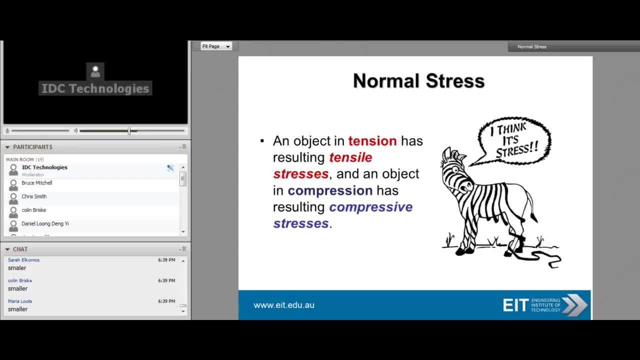 Yeah, is this going to be tensile stress here or compressive stress? do you think this zebra is undergoing? We're pulling something off him, pulling his stripes off. is it tensile or compressive stress? Oh, I think it's tensile stress. okay, all right. 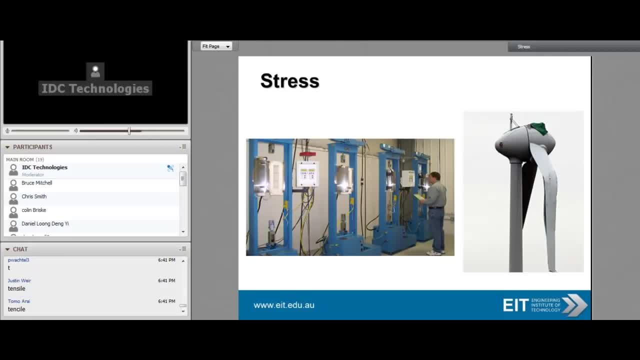 And here we've got a picture of a lab, and these are pieces of equipment called tensometers. What they do is they allow us to put samples in between two jaws, so there's a lower jaw and an upper jaw there, and then we apply a load and we stretch the tensile test. object: 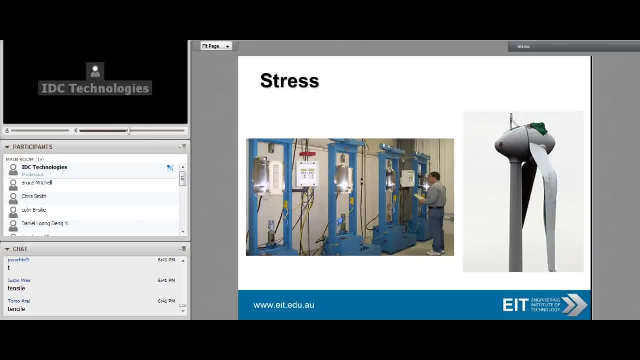 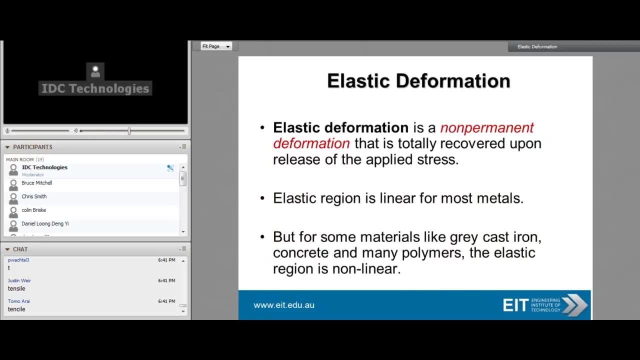 and we measure the load and the reduction in cross-sectional area and that helps us calculate the tensile strength of the material. Now I'm going to show you a sketch in a moment. I'm going to show you a sketch in a moment that explains this particular slide. 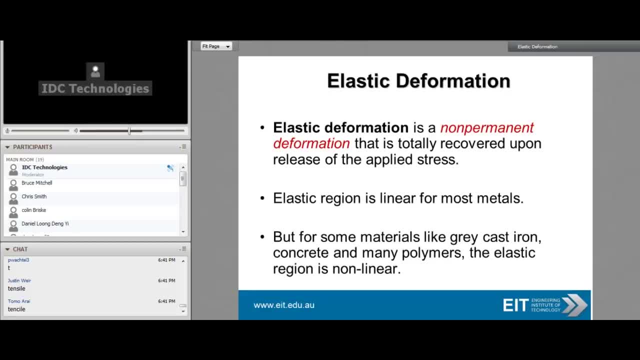 But when we talk about elastic deformation in steels or in materials, what elastic deformation means is if we apply a load to a piece of material and it stretches. if we reduce or take away the load, That piece of steel will go back to its original shape. 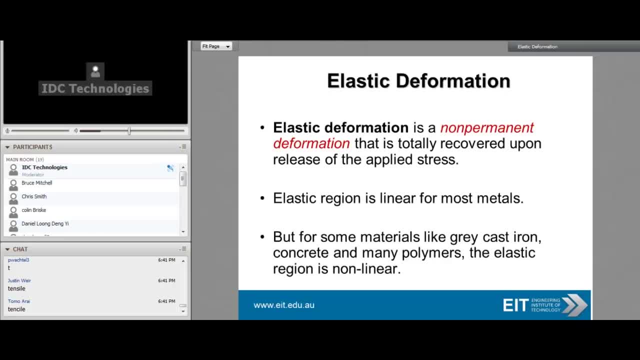 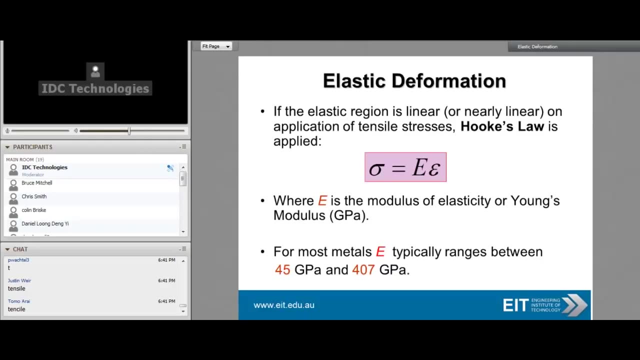 That's elastic deformation, And we're able to measure this in the laboratory doing tensile tests. So if we want to find out the tensile stress of a piece of material, then we apply this formula. Well, we know that sigma is the stress, E is Young's modulus of elasticity. that's measured. 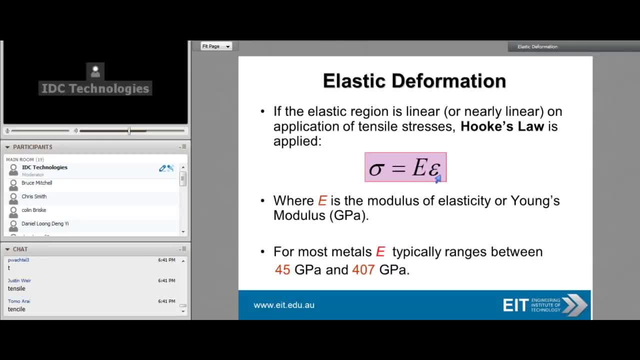 in gigapascals, and then E. this epsilon is the strain, And the strain is dimensionless. It's a change in length divided into the original length. It's a change, So it's dimensionless, And for different materials. 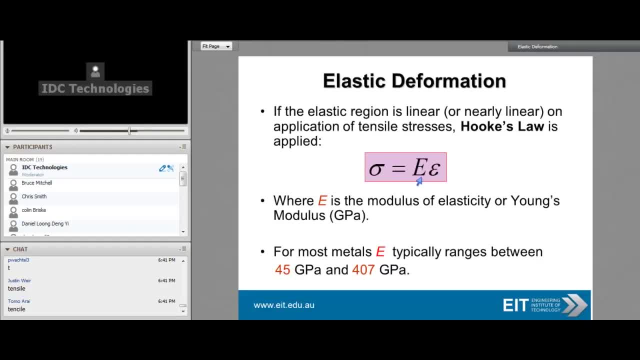 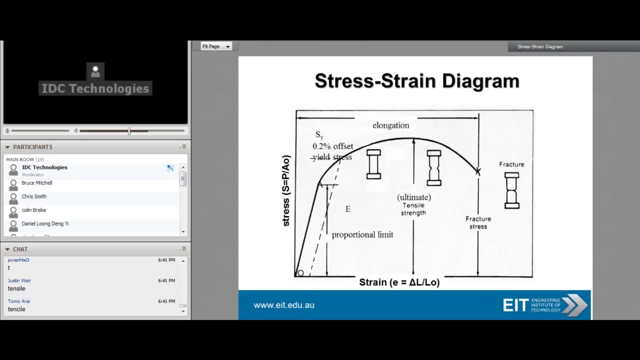 The value of Young's modulus of elasticity, capital E here can vary anywhere between 45 gigapascals right up to 407 gigapascals. It really depends on the material. Now here we've got a stress-strain diagram and there's strain. 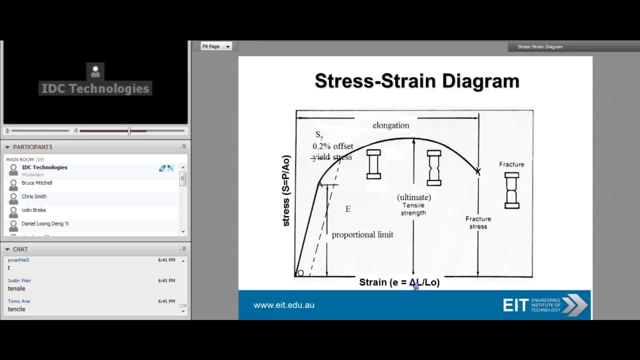 This is supposed to be little epsilon. You can see that it's a change in length divided by the original length. That's why it's dimensionless. And here's our stress: That's load divided by cross-sectional area. So if we look at this solid line of this curve, this is a tensile test on a piece of material. 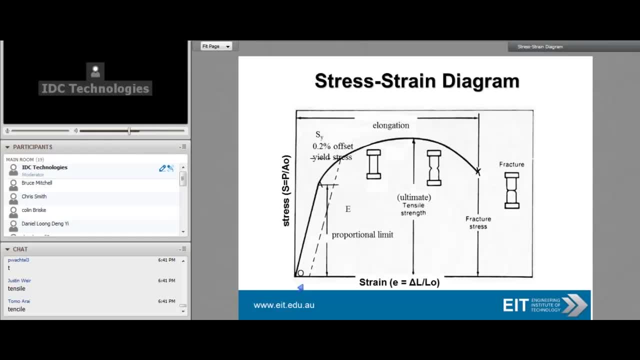 where we're measuring stress that we apply against strain. That's the stretch of the material And here you can see a sample shape of a sample. Now In this region here where we've got a linear relationship between stress and strain, this 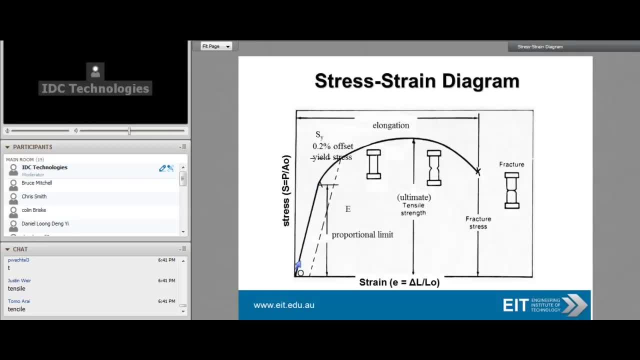 is called the limit of proportionality. In other words, stress is proportional to strain. It's linear, It's linear. Then we get to a point here that we call the elastic limit. Now, in other words, elastic limit is that stress applied to the material. 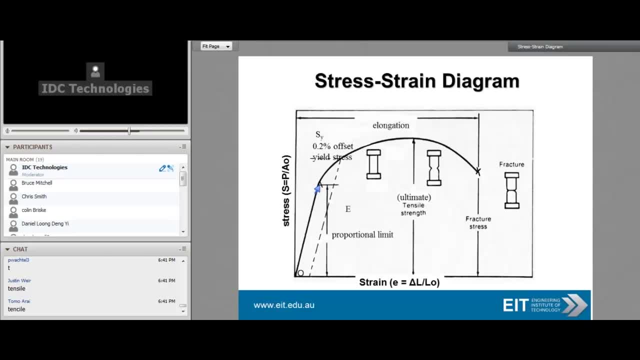 That will, when it's removed, allow the material to go back to its original dimension. Once we get above that limit, that tensile stress limit, we get what we call plastic deformation. So in other words, if I released the stress, if I released the load, my tensile test object. 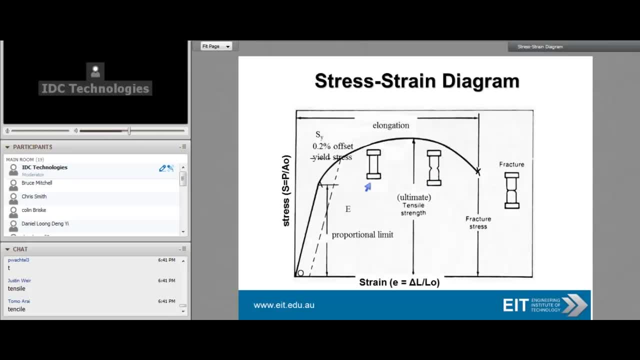 here would not go back to this original shape. And what happens is we get something called necking And you can see we get a reduction in diameter of the tensile test sample. And what's interesting is that here we get something called the UTS, the ultimate tensile. 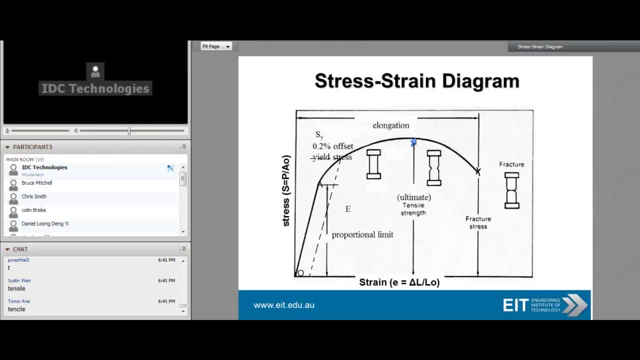 strength Once we get past that UTS point. look what happens here. I don't have to apply any more load. The material is saying: oh, that's it, That's it Well, goodbye, I'm failing. And then we get fracture of the tensile test sample. 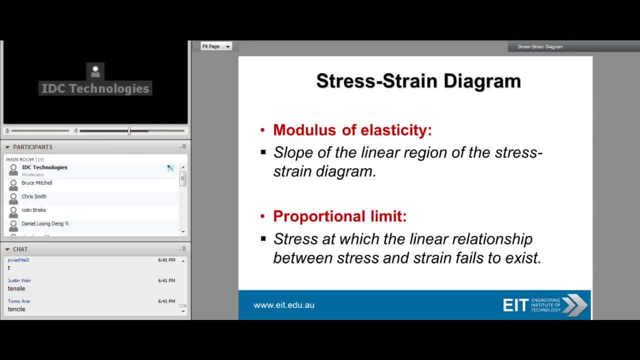 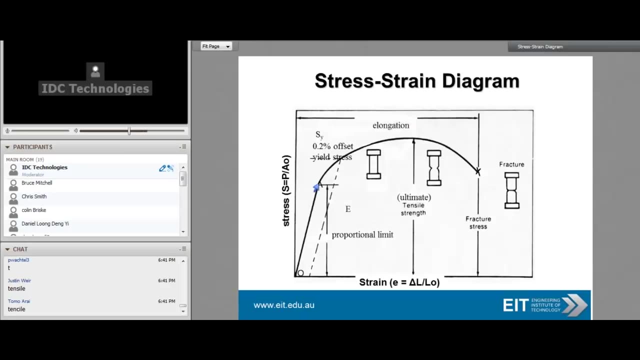 And I just want to show you in a moment what those look like. So the proportional limit is the stress at which the linear relationship between stress and strain fails to exist. That is the limit of proportionality, or proportional limit as they have been, And that's what they have on this slide here. 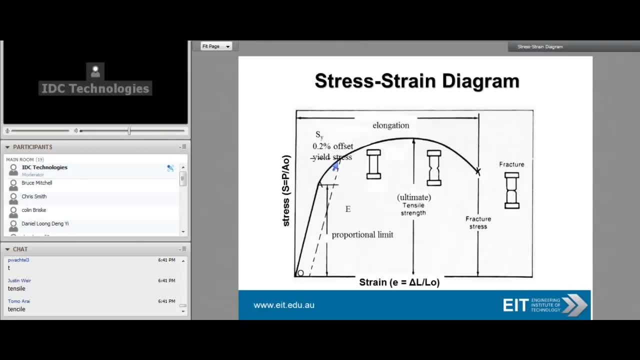 Once you're past that point, it's the point of no return. Now, engineers, when they design, whether it's a bridge, whether it's a rope for a drag in a quarry, they're always designing to make sure that we never, ever stress a material. 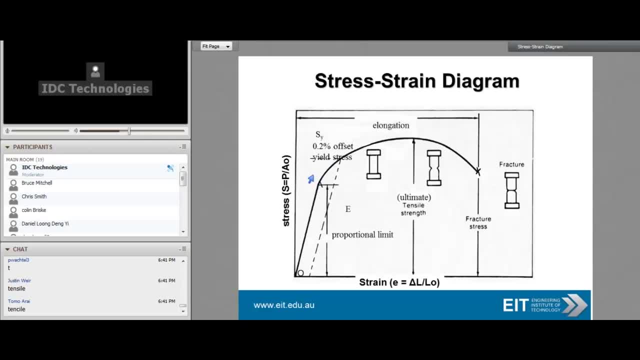 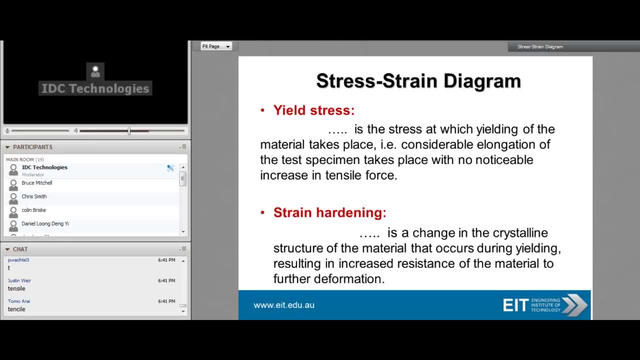 past this point here, Because that can lead to failure. Now yield stress I've mentioned before. that's where we get yielding of the material And then we get plastic deformation occurring. Strain hardening is: if you look at the sample you could see that the grain structure you 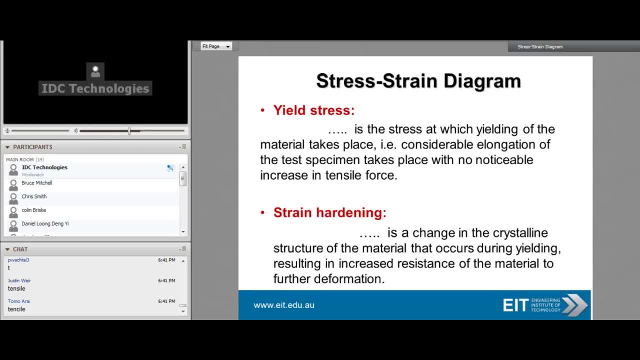 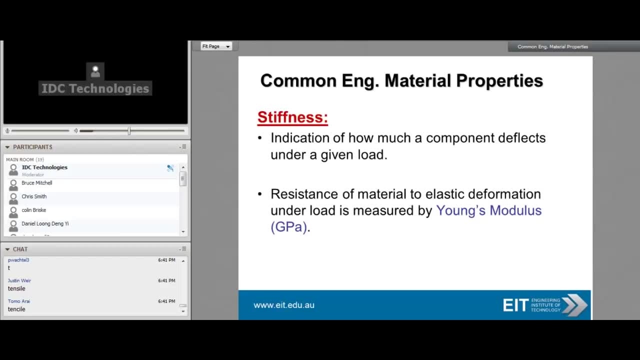 know, under a microscope you could see the grain structure of the material is actually starting to change, And that's what's doing the damage. Okay, So let's talk about engineering material properties for a moment. Stiffness: that's how much a component will deflect or not deflect under a given load. 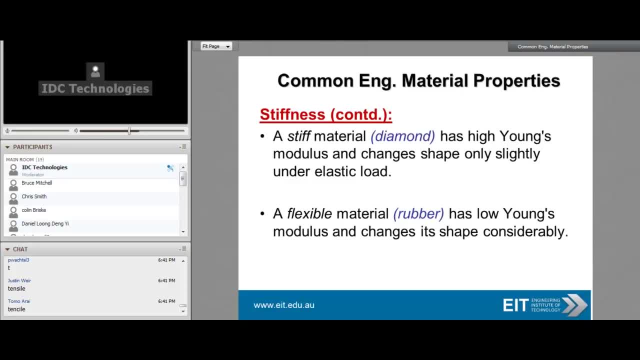 We're given a stiff material here. diamond Diamond does not change under very, very heavy loads. Rubber, on the other hand, it doesn't take much to change the shape of a piece of rubber. It doesn't take much to change the shape of a piece of rubber. 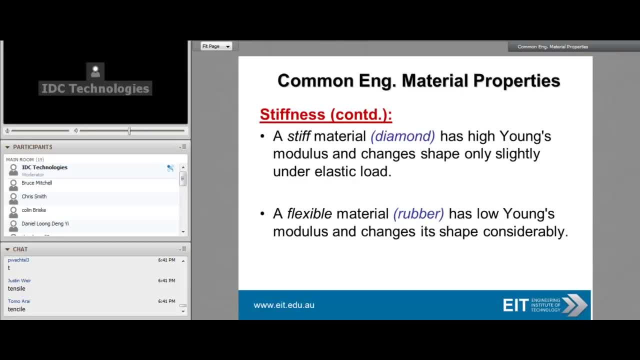 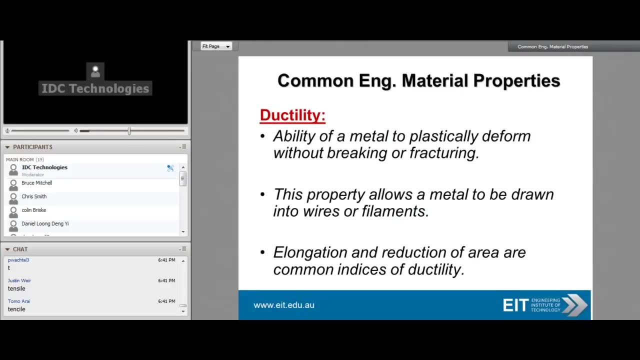 It doesn't take much to change the shape of a piece of rubber. So diamond would have a very, very high Young's modulus of elasticity And rubber, of course, would have a very, very low modulus of elasticity. Stoptility: that's defined really as the ability of a material to be drawn into wires. 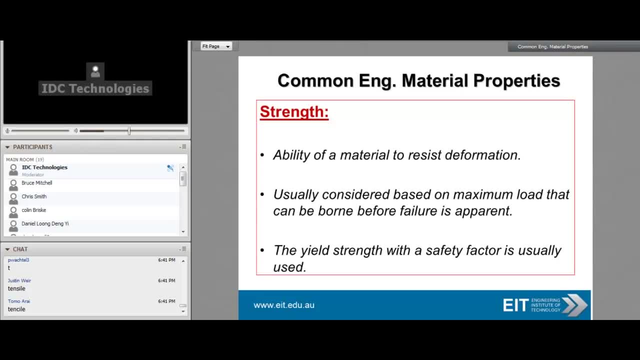 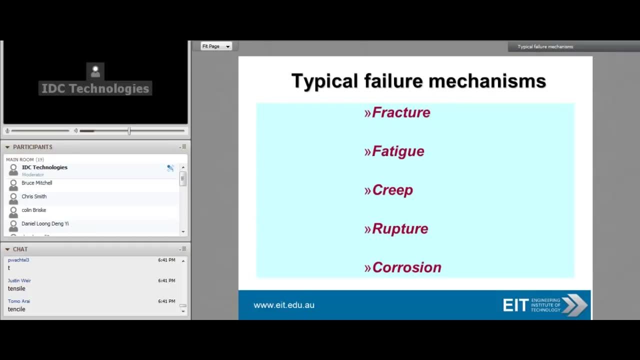 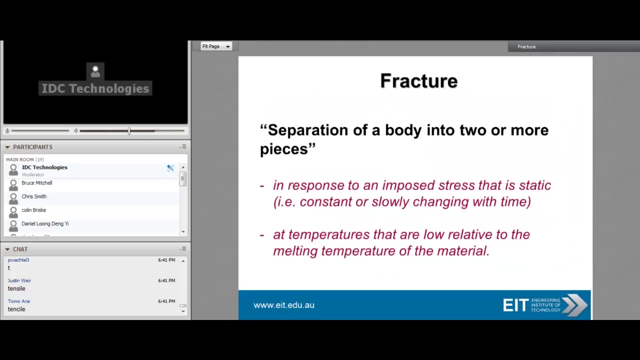 Strength, The strength of a material is the ability of the material material to resist deformation. now, when we're talking about failure mechanisms, engineers, when they're designing equipment, have to take all of these five failure mechanisms into account when they're designing equipment. well, fractures, defined quite simply as a separation of a body into two or more, 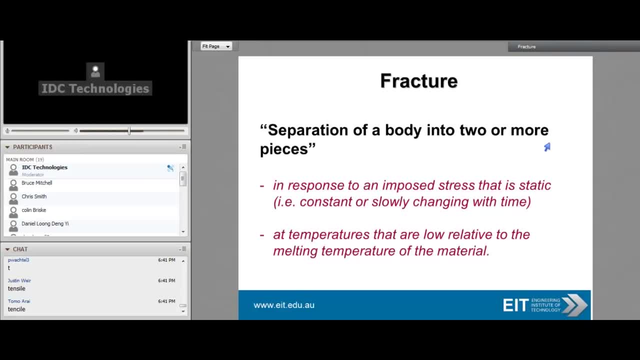 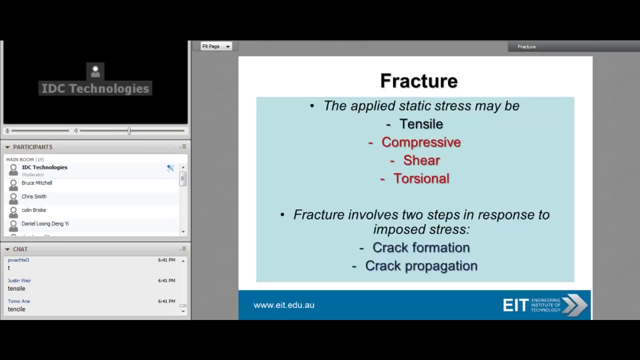 pieces and, let's hope, if we design something that we never ever see fracture occurring now. fracture can occur under conditions of compressive stress, shear stress and torsional stress, and there's definitely two steps in the process that occurs before we have ultimately a fracture on our hands and that is the formation of 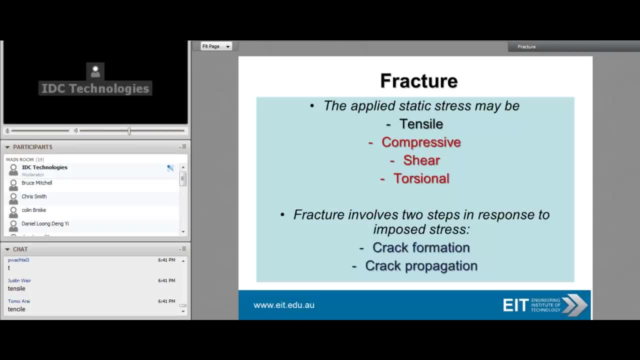 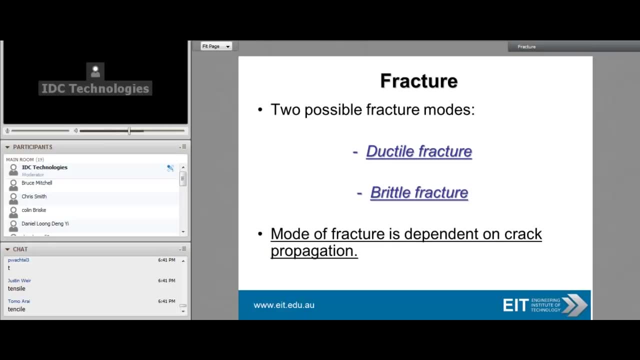 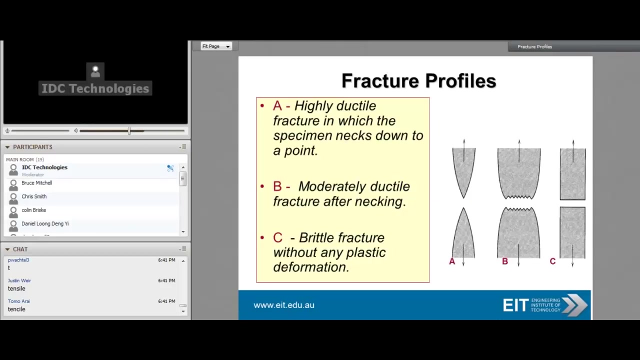 cracks, and then the propagation of cracks, and we've got two possible fracture modes: this fracture occurring under ductile conditions and fracture occurring under brittle conditions. now let me show you the samples of these tensile test objects that I was talking about before. imagine those tensile test machines with tensometers producing a. 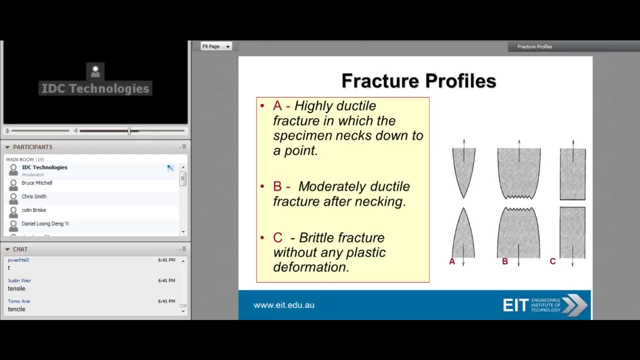 load and on on samples until they're actually fracture. this would show you the different samples of different materials and the fractures that we get, depending on the ductility of the material, of the, of the, of the sample. here we can see that we've got necking. that's really. 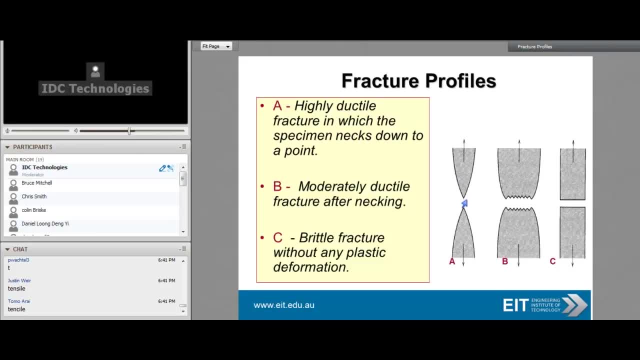 really visible. so, in other words, this material has stretched and stretched, and stretched and then bang it's, it's broken. this is indicative of a very highly ductile material, something like copper, something like aluminium. here we see there's been a definite reduction in the size of the sample up to the point of fracture and then at the point of 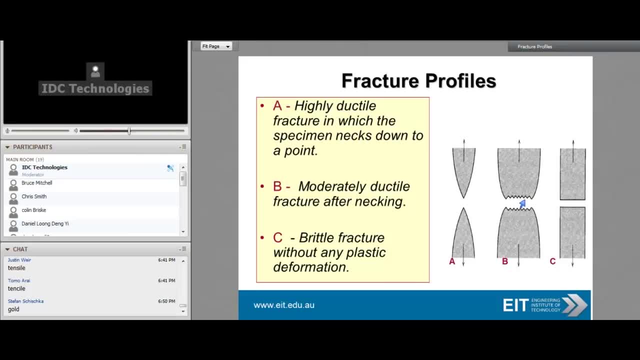 fracture. now we can see this sawtooth pattern here, where the samples are torn apart from each other. so this is what we call a more great ductile fracture. you see that in some stainless steels, for example, and then on here on this particular one. here we've got the 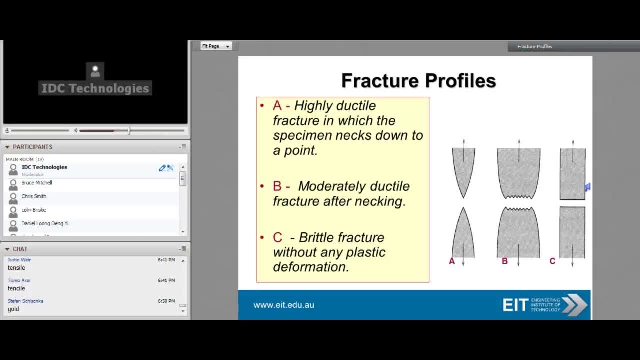 brittle fracture. you can see no reduction in cross-section here. and what happens is we load the sample, it doesn't stretch. we load the sample more, it doesn't stretch, we load the sample more, it doesn't stretch. and then what happens is we reach the ultimate tensile strength of the material. 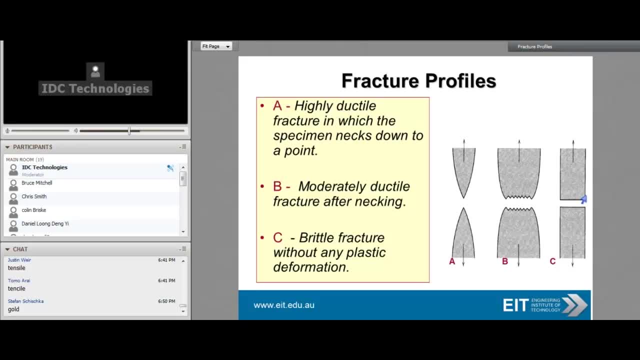 without it having stretched and then bang, it just gives way, and this is indicative of a highly brittle material. any ideas what that might be? well, can you think of a highly brittle metal, for example? highly brittle metal, yep well, cast iron is a very, very common material that is very brittle. 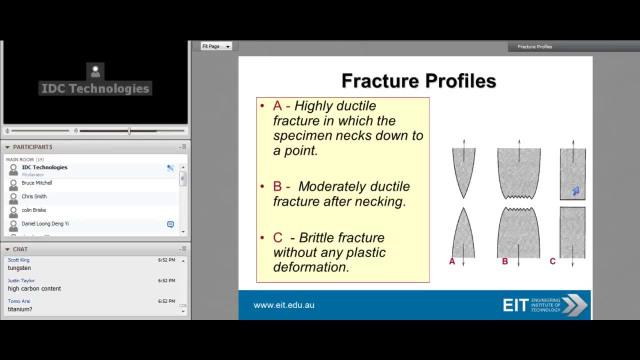 tungsten, you said, is as brittle as well. titanium, mmm, I think in titanium you're going to see, this one is moderately ductile, tiny, tiny is. is that high-speed steel? yeah, I think it's going to be. it's going to be there on the, on the, on the brittle fracture brass- no, you will see some necking on the sample before it. 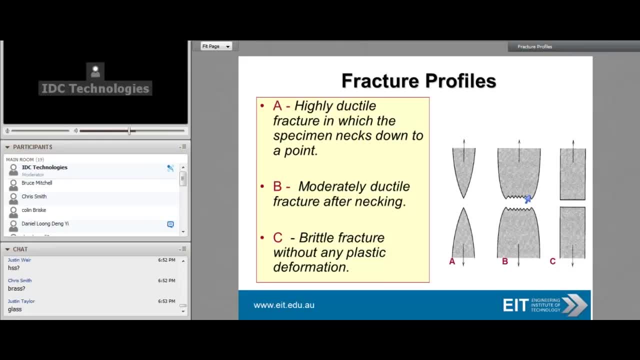 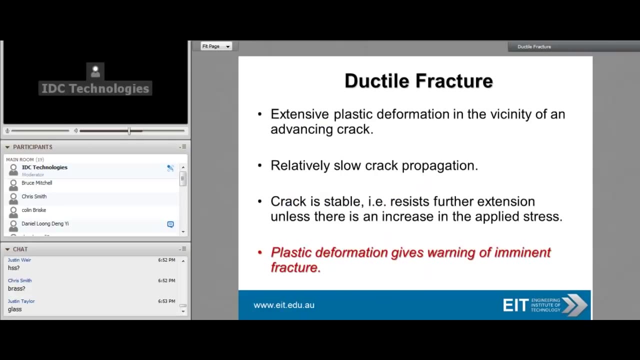 gives way. so brass is is moderately ductile glass. well, it's definitely brittle. ever stretch, try to stretch a pane of glass? I haven't, but it would be interesting to see if you could. yeah, yeah, glass is definitely brittle. now with ductile, the metal is not solid. brass is stable all the way down because the process is. 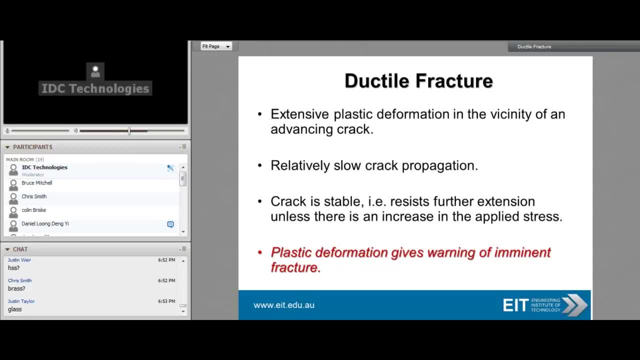 we get a very slow crack propagation. if we reduce the load then the crack becomes stable and it's not a great situation to be in. but we won't. we won't get any any any fracture occurring unless we reapply the load and carry on doing that until we get to a certain stage where we've got that typical fracture. 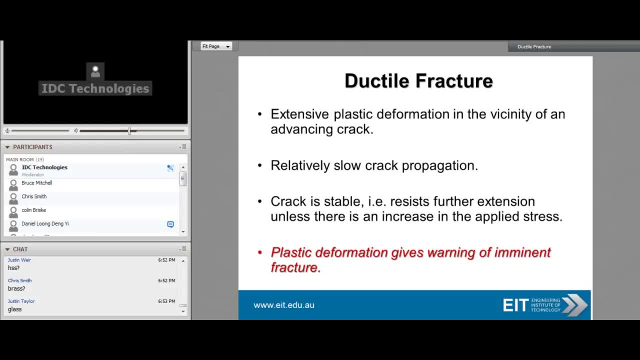 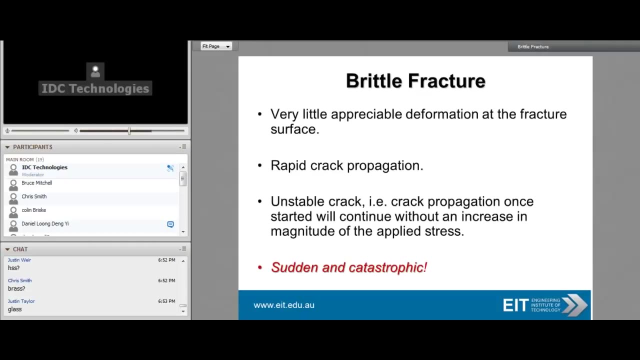 plastic deformation, where the material has visibly stretched and we know around the corner, fracture is just waiting to happen. So that's ductile fracture, With brittle fracture it's the other extreme. What happens is you get very, very little, if any, deformation at the 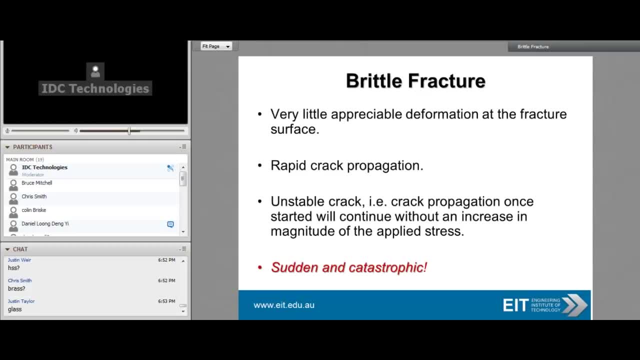 fracture site And you know, as I said before, we apply a load, keep on applying it, keep on applying it and then bang, it goes. And it goes very, very suddenly. You get rapid crack propagation And a brittle fracture is extremely quick And it can be very catastrophic. 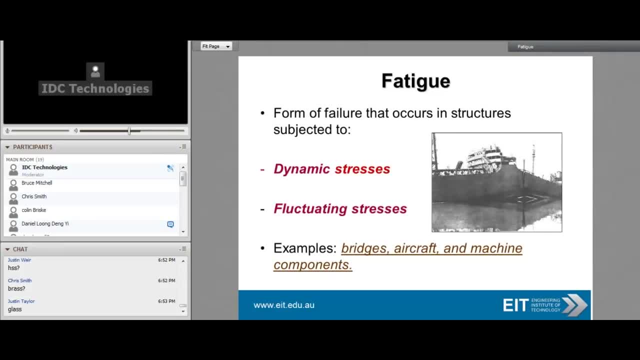 Other failures that we can see in construction are dynamic stresses and fluctuating stresses. This is where the stresses are going up and down and the dynamic stresses are going back and forth, And what's happened here in this pretty little picture, is this boat has broken in half. It's broken in half due to fluctuating stresses. I'm glad I didn't design. 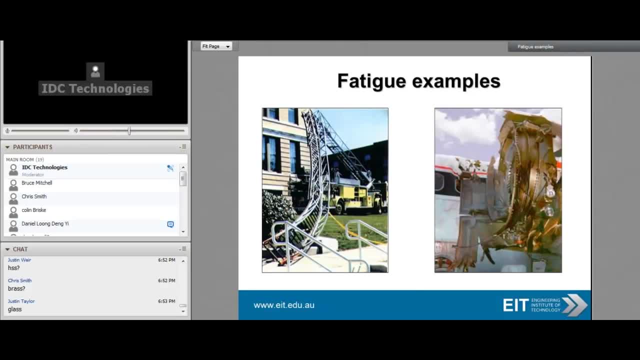 that. Here's some examples of fatigue. We've got a truck with a ladder on here And, oh dear, the ladder has broken and, okay, it's bent as well. How about this as an example of fatigue? We've got a jet aircraft engine where the 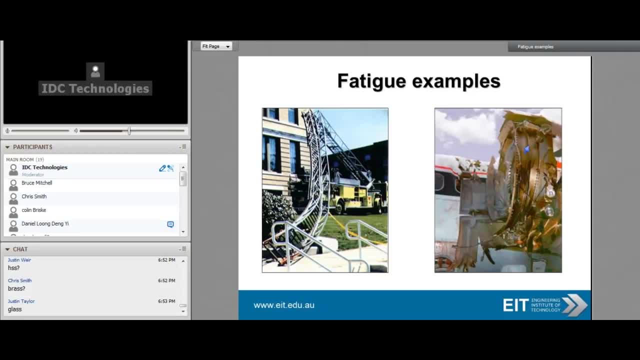 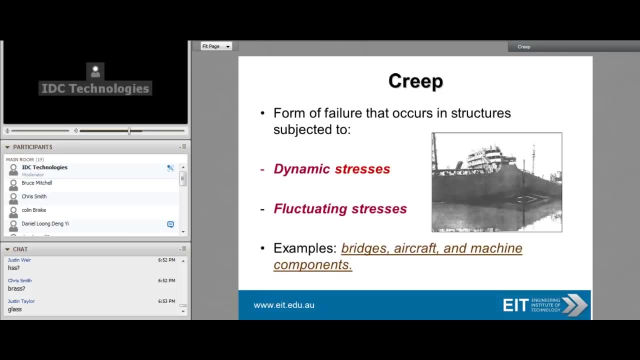 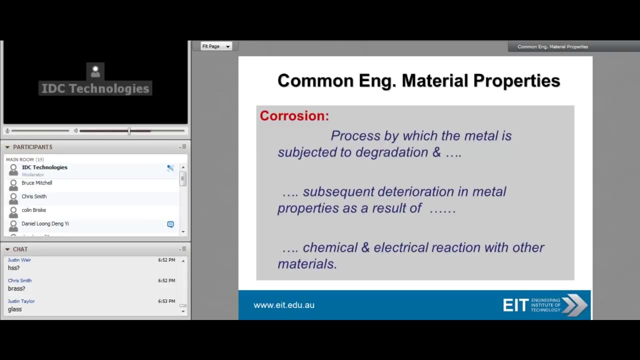 blades of the jet engine flew apart and they just burst the casing of the jet engine. These are things that people- engineers- have to design out, So we've really got to be aware of these things. but also using these different techniques- senators have MicroScreen, Caraышi and Trinity have generation steps and爸爸 لست hacks that are all important for their design. These are things that engineers have to design out, And so we've got to really be aware of where these went in the past. This equipment is justency, and I do give you the information there. They are just a matter of what you're going to need to do. There are some patterns, Most of these surprises, and I hope you do so. make the measurements for a car like- And I'll also talk about how youores have to guide the of stern pasteurization And then make the 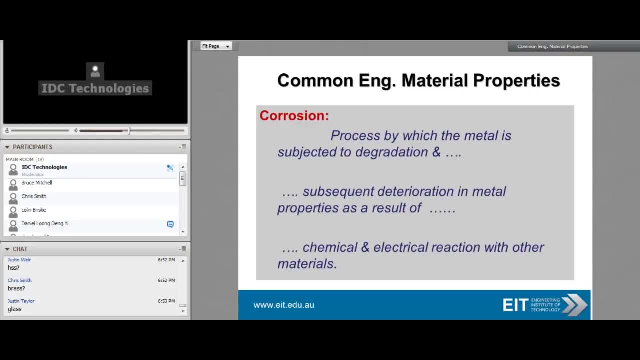 these things. Another form of stress is corrosion. Corrosion, basically people, is what. Can somebody give me a definition of corrosion, but a very, very simple one? Okay, we've got some pretty ones To me. corrosion is a loss of material due to a chemical and. 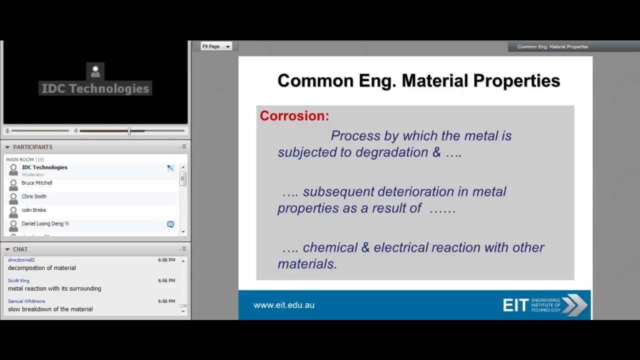 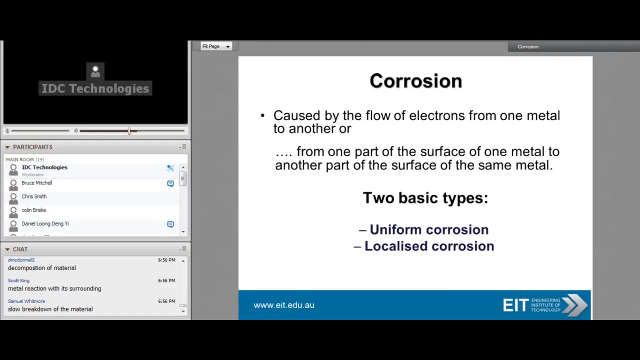 electrical reaction. It's a loss of material. It can be gradual or it can be rapid, but it's a loss of material, And if we lose material, then we lose strength. Now there are two types of corrosion that we're going to look at in this webinar. 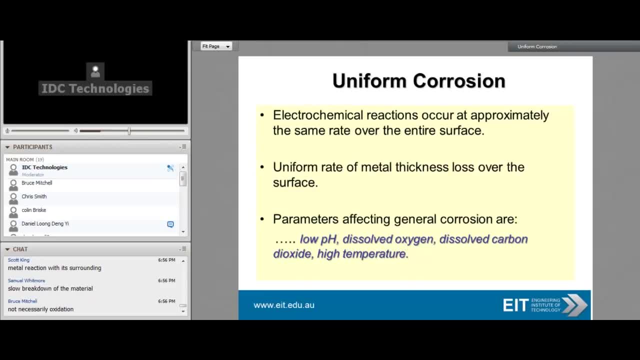 That's uniform and localized corrosion. With uniform corrosion, as the name implies, it happens all over the surface and basically the corrosion rate is the same over the surface of the material And things that can affect corrosion uniform corrosion are low pH. 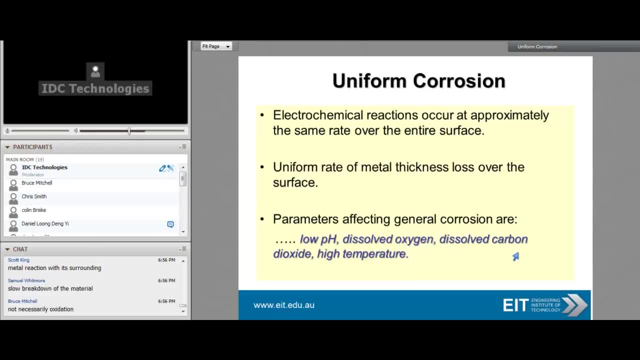 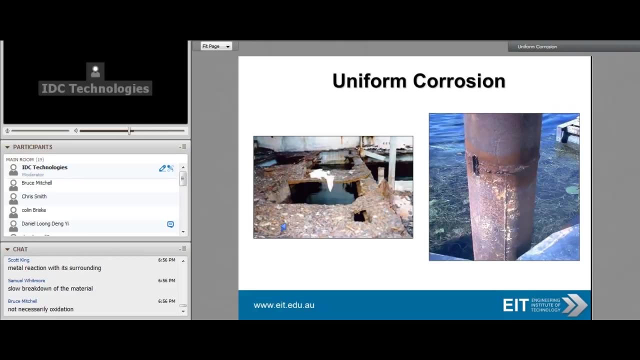 things that are very, very acidic: dissolved oxygen, dissolved carbon dioxide. Another one here is high temperatures. High temperatures can accelerate corrosion, And here's some examples of uniform corrosion. You can see this floor, this steel floor has been eaten away and you can see the corrosion. there is uniform. I don't know who was standing. 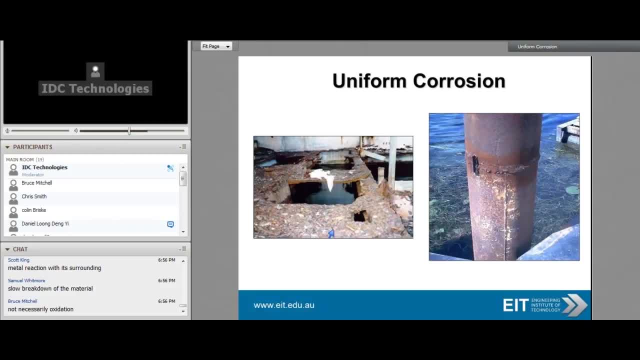 there before that gave way, but anyway, you can see that that's happened here in this construction site. And another example is where we've got a pillar in seawater And you can see where the high tide is here, can't you? Okay, there we've got a good example of uniform corrosion. 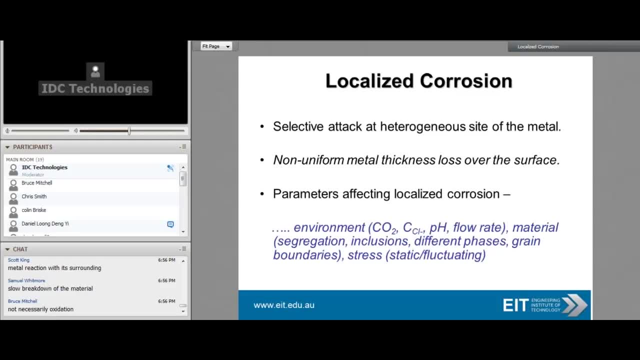 Localized corrosion is where we've got non-uniform loss of material over the surface of the component, And things that affect that are carbon dioxide, calcium chlorides- especially in stainless steels that contain calcium chlorides, and that can affect local corrosion. And here 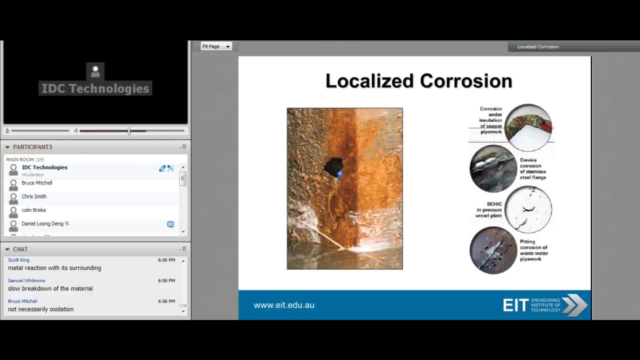 we can see an example of localized corrosion. This is so localized here that it's actually gone right through the material, And there's some examples here on the right-hand side here of localized corrosion. We've got something called here SOHIC S-O-H-I-C. Does anybody know what SOHIC is? Well, the 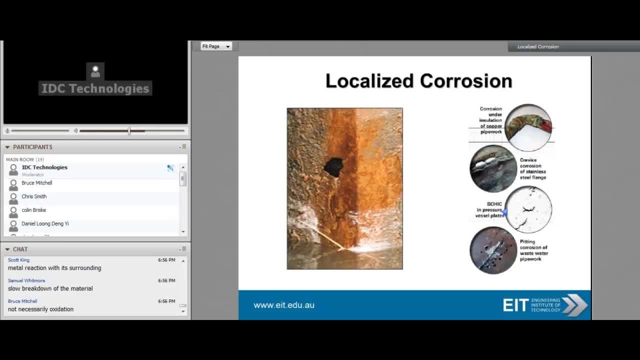 letters S-O-H-I-C stand for stress-oriented hydrogen-induced cracking. It's a fancy name for what happens when we get hydrogen sulfide corrosion. You know hydrogen sulfide is the stuff that smells like bad eggs. If you've ever been in a refinery you can smell it often That's sulfate. I'll say it in English: hydrogen. 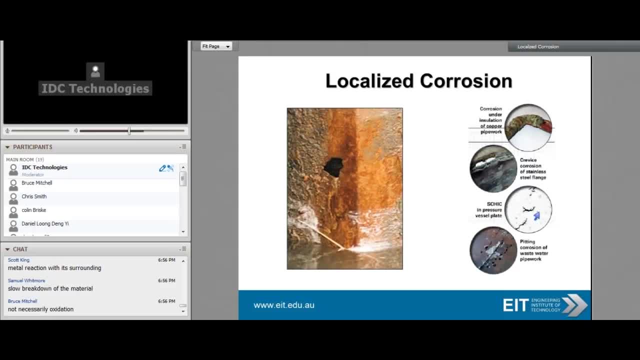 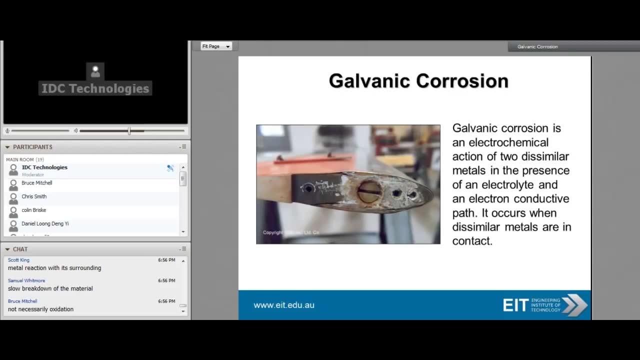 sulfide- attacking weak points in the material here- And galvanic corrosion. Can anybody give me an example of where galvanic corrosion occurs? No hint, but I think the name might give it away. Where do you think galvanic corrosion? 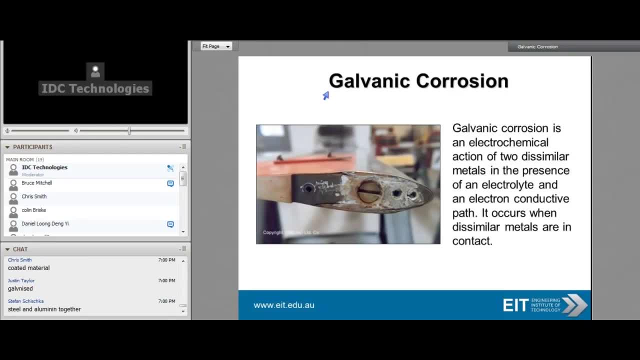 occurs In steel and aluminum? Yes, that's for sure. What else have I got? Aluminum and stainless steel bolts: Yes, Underwater on ships' hulls, The propellers- Yes, Good example. What else? Aluminum and stainless steel bolts: Yes, Underwater on ships' hulls, The propellers- Yes, Good. 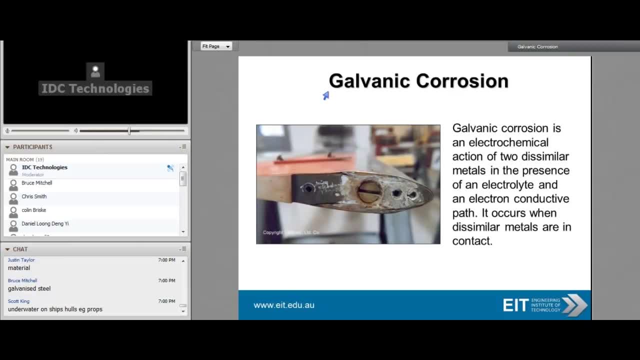 example, Aluminum and stainless steel bolts: Yes. Underwater on ships' hulls: Yes. Good example, Bruce. brilliant example. You got what I was hinting at there: Galvanized steel people. That's where it happens there. So in galvanized steel, for example, the zinc which is the 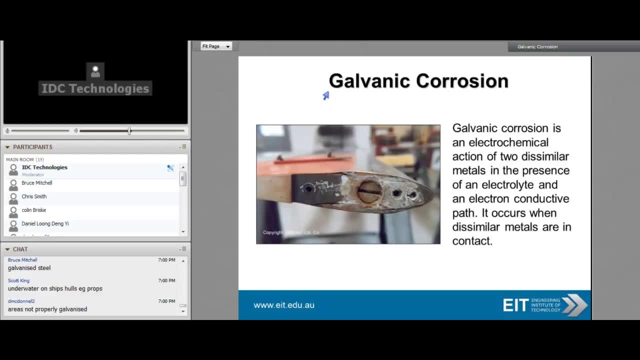 galvanizing sacrifices itself to protect the steel and we've got two dissimilar metals in contact with each other: steel and copper. And if we looked at the galvanic series, the table in the galvanic series, we'd see that in actual fact, zinc and steel are fairly close together. 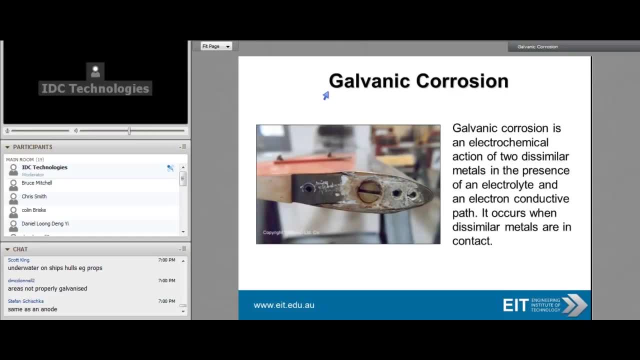 If you looked at that same table and looked at copper, now copper could protect steel, but steel and copper are further apart in the galvanic series. And what will happen is if you copper plate steel and compare the life of its ability to protect the steel, you'll find it's shorter than the zinc under the same conditions. 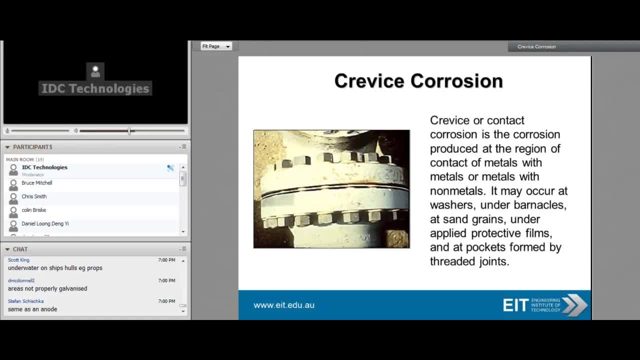 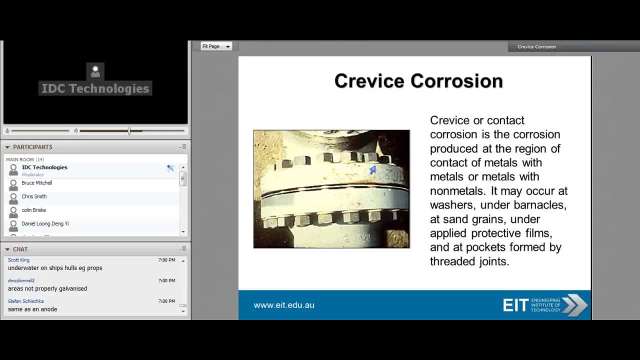 The heads of washers, and I think someone gave me an example there of aluminum and steel bolts- definitely could get that where you've got dissimilar metals and you've got some kind of electrolyte. It could be water, it could be leaked product, whatever. 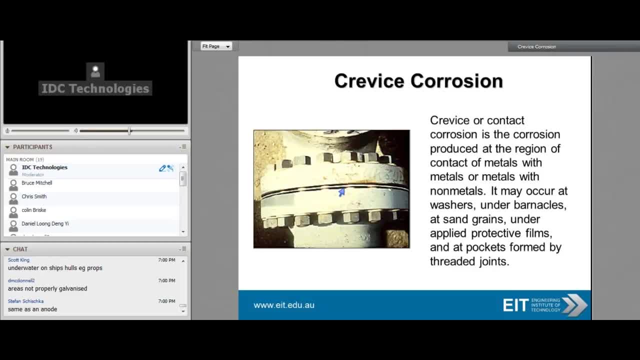 You can also get it in gaskets. You get steel gaskets that can accelerate corrosion if they're not selected as material. You can also get steel gaskets that can accelerate corrosion if they're not selected as material. You can also get steel gaskets that can accelerate corrosion if they're not selected as material. 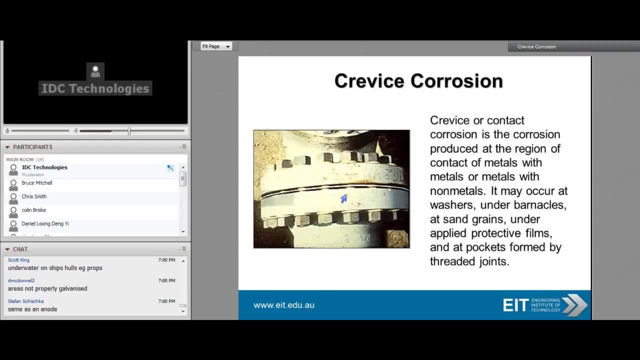 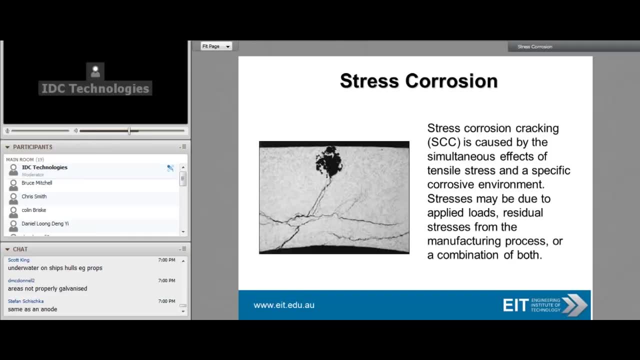 It's not selected properly And stress corrosion, cracking SCC. well, we see that in sulfuric acid tanks, where the chlorides sorry, in hydrochloric acid tanks that are made from stainless steel, where the chlorides and the acid actually attack the steel where it's been stressed. And stress corrosion cracking SCC. well, we see that in sulfuric acid tanks, where the chlorides and the acid actually attack the steel where it's been stressed, And stress corrosion cracking SCC. well, we see that in sulfuric acid tanks, where the chlorides and the acid actually attack the steel where it's been stressed. 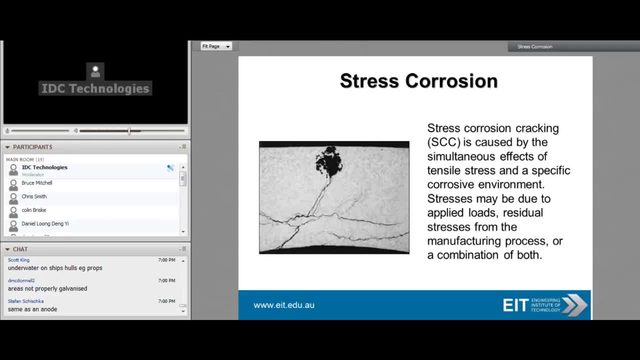 And stress, corrosion, cracking SCC. well, we see that in sulfuric acid tanks, where the chlorides and the acid actually attack the steel where it's been stressed. And you know, when a tank is being filled up it expands. so the steel is being stressed, it's being stretched, and then when the tank empties, then the steel is being compressed. 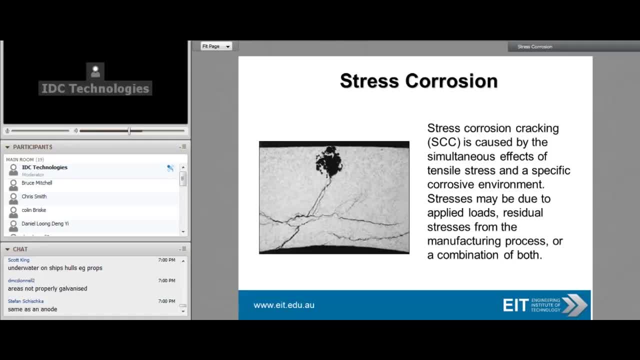 It's trying to get back to its original shape. Springs, for example. mechanical steel manufacturers, to reduce the cost of producing their mechanical seals, often make the springs out of stainless steel. Now, that's fine if you are using them on water that has very, very low chloride content. 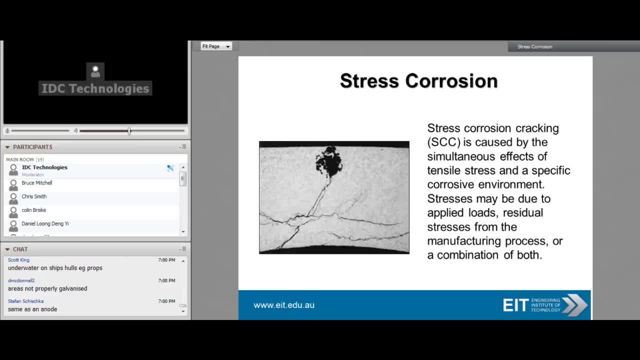 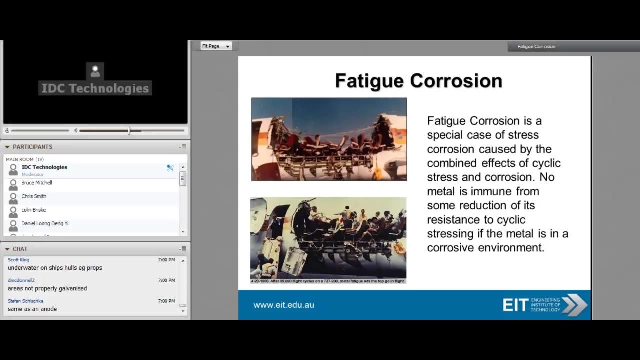 But if you've got anything that's got any significant amount of chlorides in, what will happen is that spring will crack and it will fail and the mechanical seal will ultimately fail. How about this example of fatigue corrosion? What you've got here is: 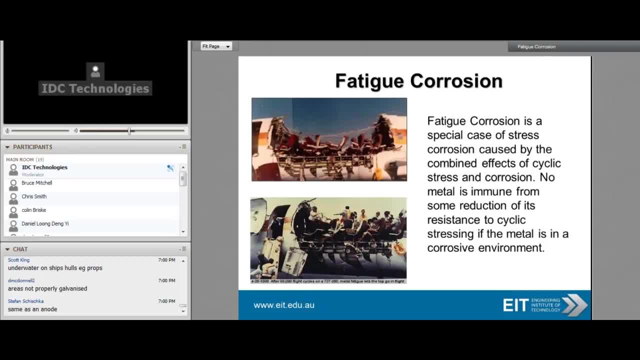 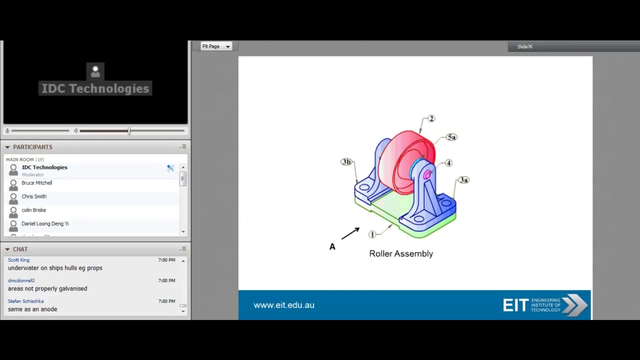 You've got the presence of stress along with corrosion, so the parts are stressed psychically, and you've got the added devil of corrosion, so that accelerates. They feed on each other and accelerate each other. Oh, and that brings us to the end. 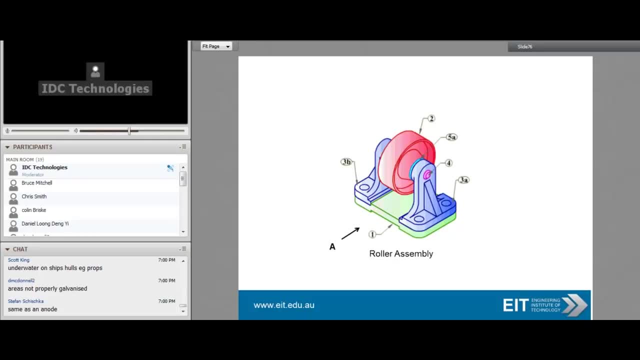 Now you'll see there's a slide here of erosion Bye. It's starting to get a little difficult. but let's just put this off for a moment and you'll see that after we've done that. I'm not going to play around with this. I'm going to take a little tease of it and I'm going to show you the look of this roller assembly. 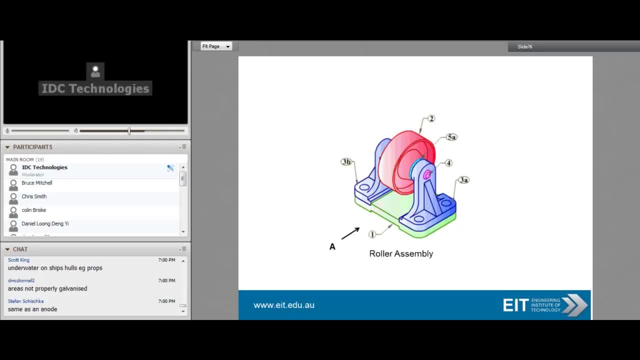 Your assignment question asks you to show an assembled sectioned view of this roller assembly. So I just wanted to explain what we're looking for in that question, because last time we ran this workshop a lot of people said: well, we don't understand what you're looking for. 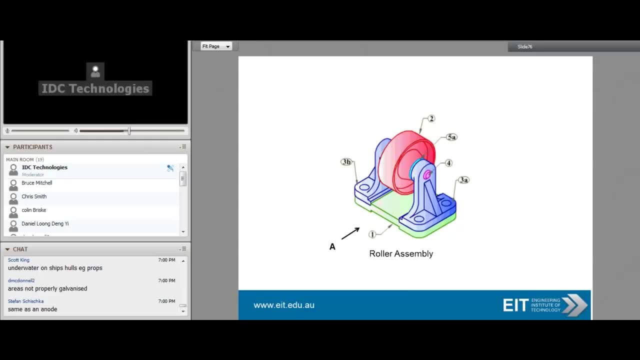 What we're looking for is your assignment question, So let's give it a little peek here. I'm going to show you the result It's going to turn out to be. is you to do as a drawing of this assembly sectioned? so imagine i took a hacksaw. 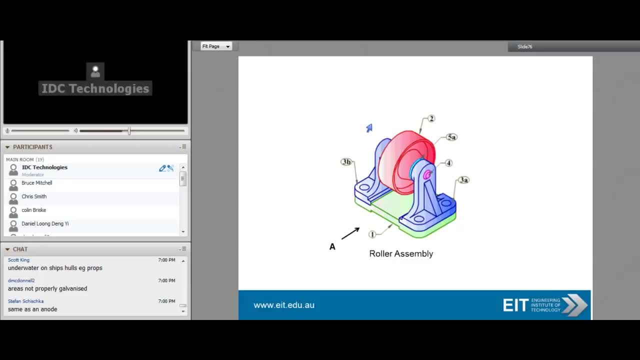 and i cut down the center of this roller along this axis and i cut right through there and then all the way down through there, so i cut this whole assembly in half, from top to bottom. what we're looking for is: what would the view look like with this thing sectioned, with this thing cut in half? are you all with me on that? that one? 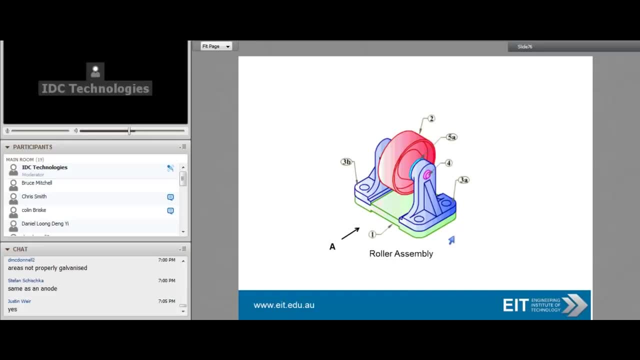 is that? is that, clear people, what we're looking for? great. well then, good luck with that question, and i'm glad you're. yeah, yeah, justin, it doesn't have to be done. doesn't have to be done on computer, um, a hand-drawn sketch, as long as it's clear. 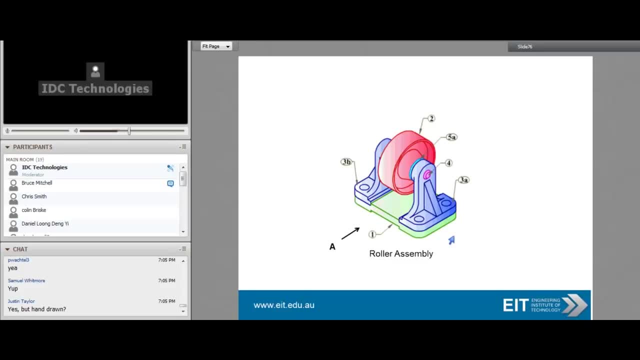 and it shows the components: um, you can draw it by hand. what we're looking for, people, is your: uh, you can. you can draw it by cad, if you want. um. and when you say bruce, what format do you want to send, just please explain. well, it'll be it. well, it remember it'll be uh. well, you can do it in pdf, you can do it on. 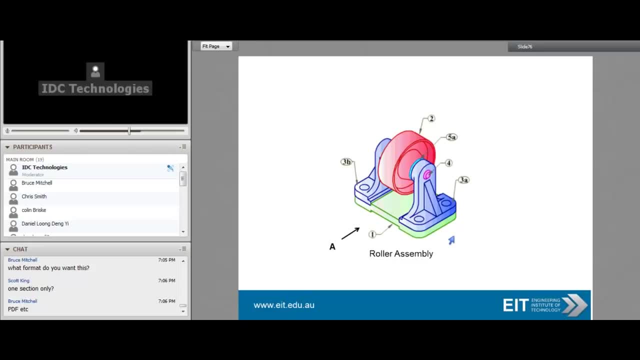 whatever, remember, it's going to go on your exam paper. so, um, if you're going to do it, um, you might want to do it by hand, um, and then, uh, then scan it and bring it, put it into your, into your exam paper, whatever, whatever suits you at the end of the day. 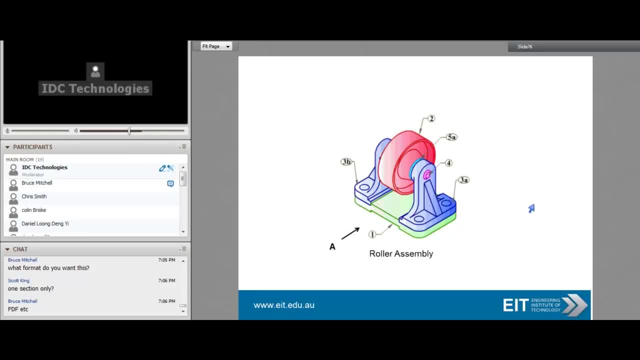 what we're looking for is your understanding of what this assembly would look like if we cut it in half and we looked at it from the direction of letter a. so you've got one section. it's cut all the way through there, but don't forget, it's one drawing. it's one drawing, but 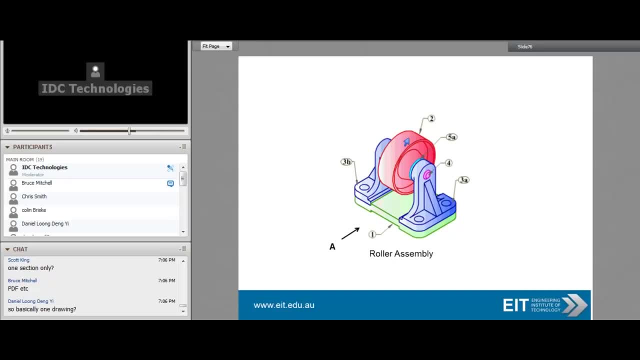 it's going to show different components, sectionalized, isn't it? and that's the only help hint i'm going to give you on this. the rest you're going to have to think through. so it'll be one drawing showing a sectionalized view of this roller assembly. 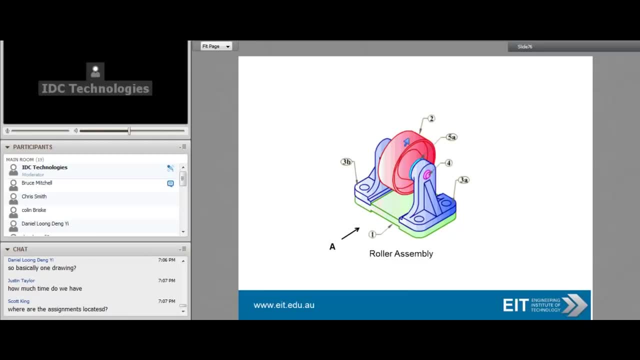 um, people, the, the. i'm just the lecturer. um the. um, uh, assignments will be given to you by eit. um, and you'll find them normally on moodle. okay, people? um, are there any questions on anything we've done in this module that you'd like to ask now? um, i usually put my email address on the very, very last slide, um, but 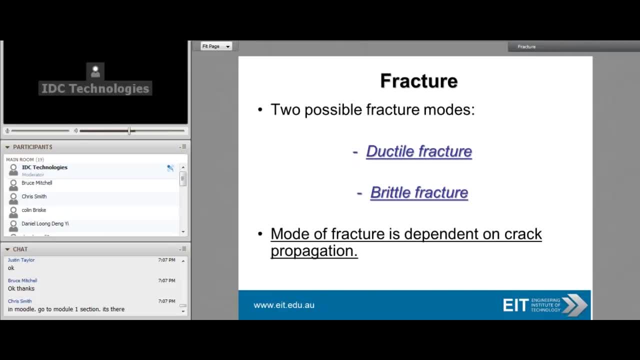 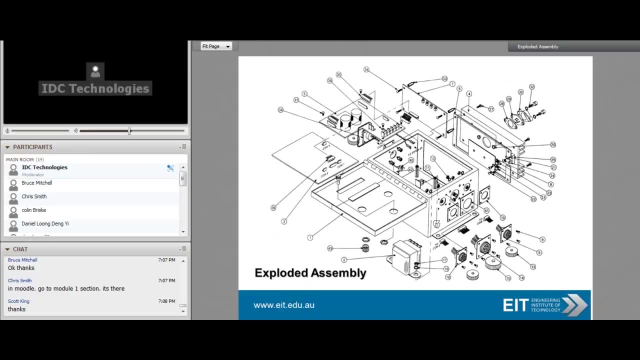 for you guys that uh. well, actually you'll get all of these slides on moodle, uh, but if you want to make a note of my email address, if there's anything that you'd like to ask me, um, apart from the answers to the to this, the assignments, um, you're more than welcome.